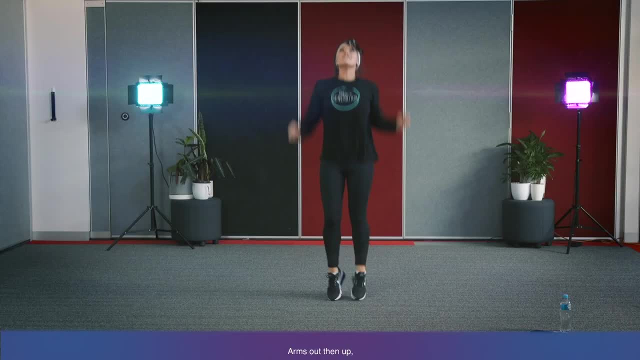 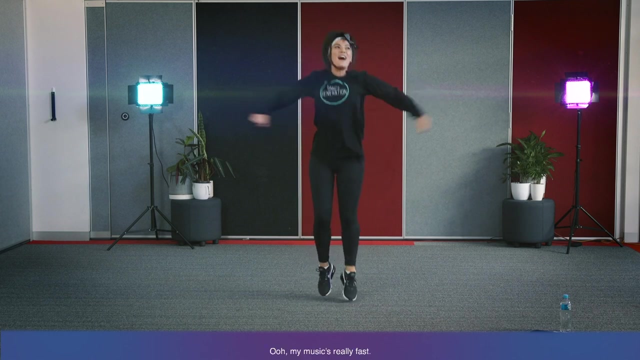 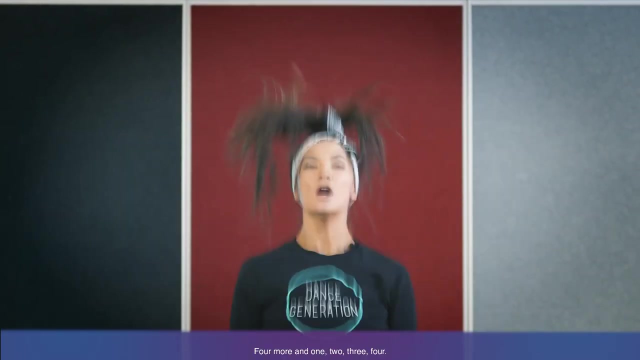 Good, Good, Good, Good, Good, Good Good. My music's really fast And star jumps. Let's go, Keep going. Four more, And one, Two, Three, Four, Let's punch it out to the side. 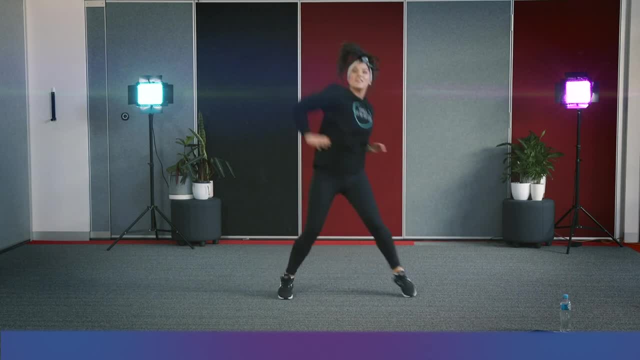 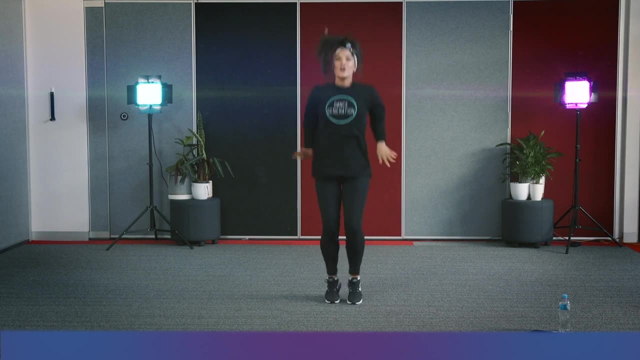 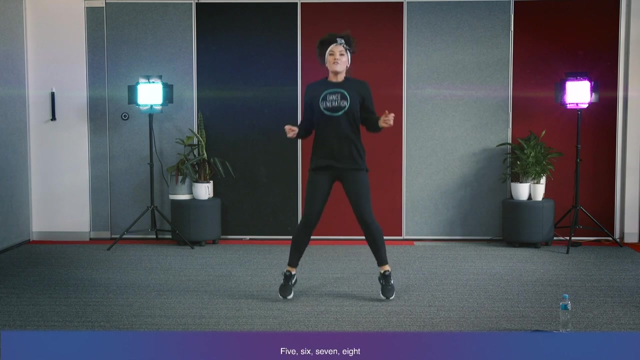 Are you guys following me? All right, Just jumping on the spot. Good, Good Should be warming up now. Take your feet out. Five, Six, Seven, Eight, And in Two, Three, Four, Five, Six. 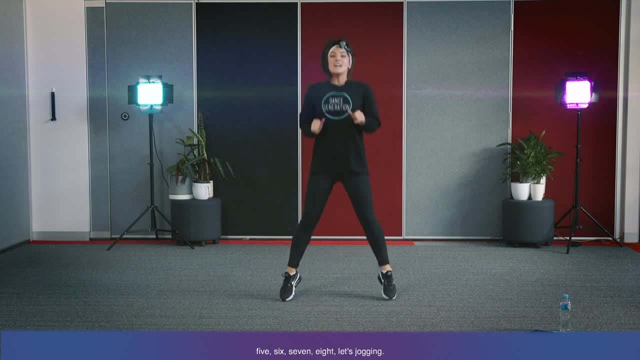 Seven Eight And out: Two, Three, Four, Five, Six, Seven Eight. Let's jogging, Keep going. Let's do a step Together, Step Together, Step, Jumping it out. Good, Keep it going. 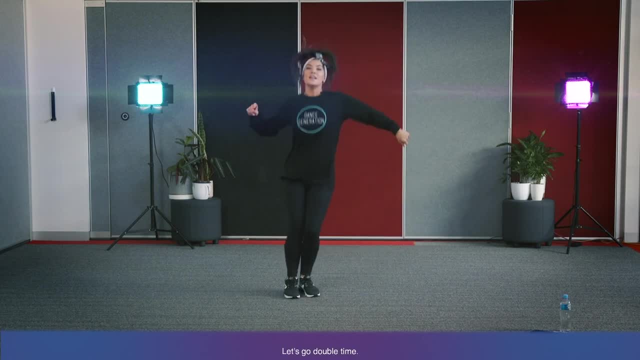 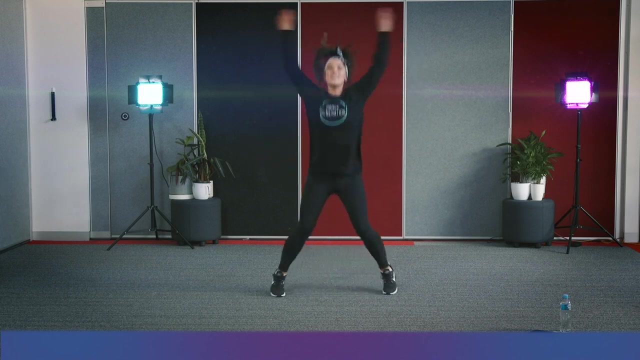 Really good guys, Let's go. double time: Let's go. And I'm getting warm now, All right, Last lot of star jumps- Really good. Four more, Let's go. One, Two, Three, Four, Reaching up. 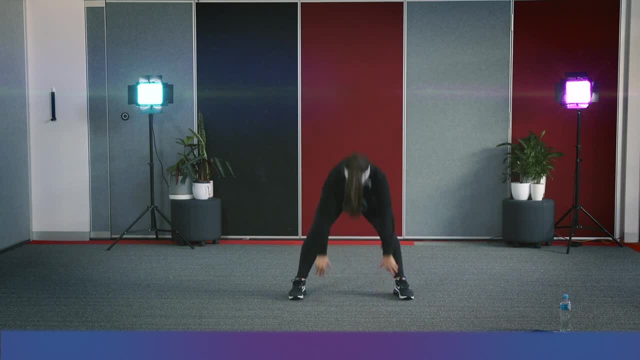 Bend your knees. Touch the ground And up, Up, Keep going Side on Looks like up Bend your knees. Good, Four more. One And two And three And four. All right, Give your legs a shake. 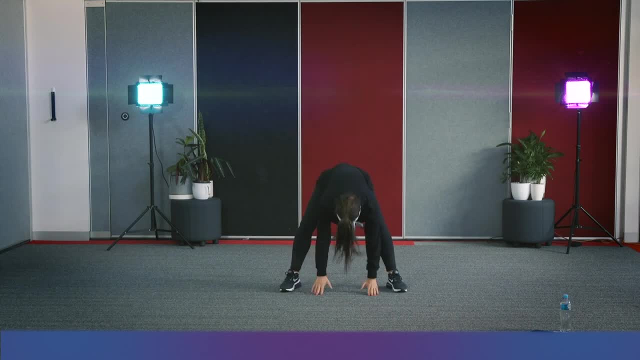 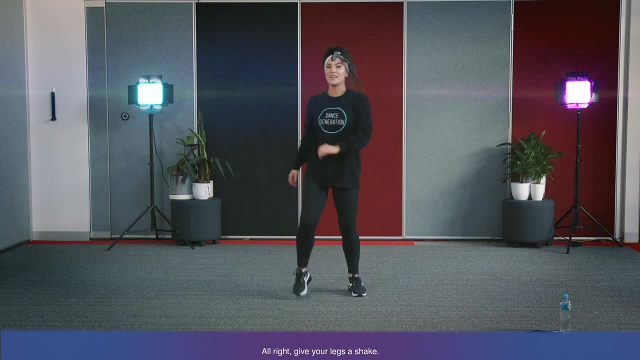 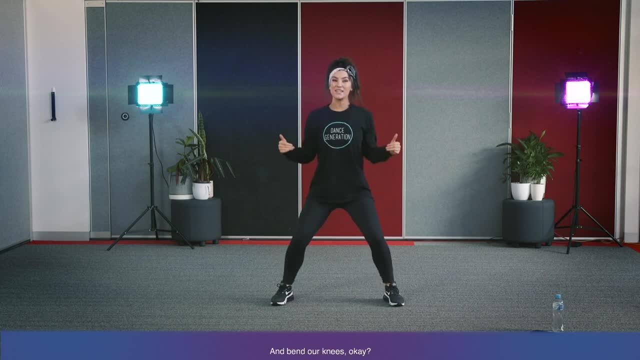 Let's tuck our feet wider than our shoulders and bend our knees. Okay, So we're nice, steady stance. Let's do some hips Good. Keep your knees bent, Just your hips Good. Double time Let's go. 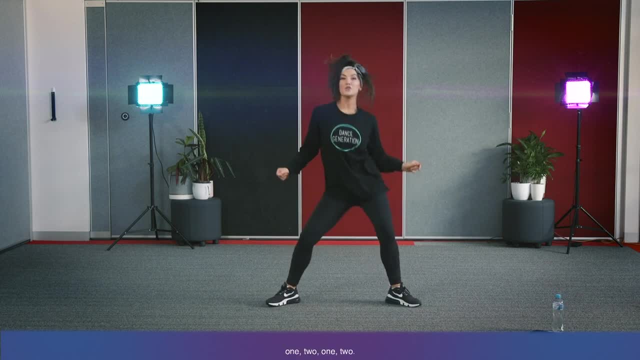 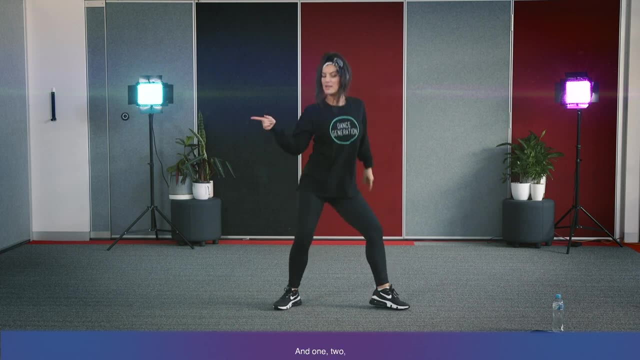 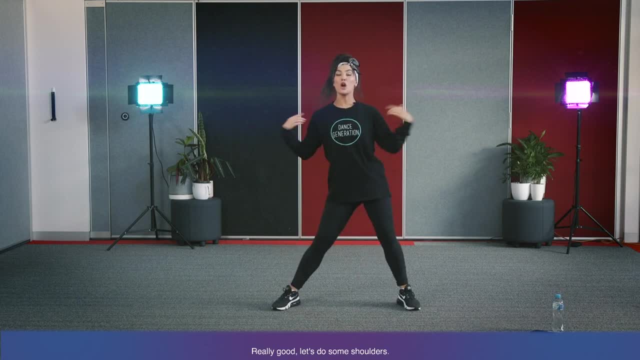 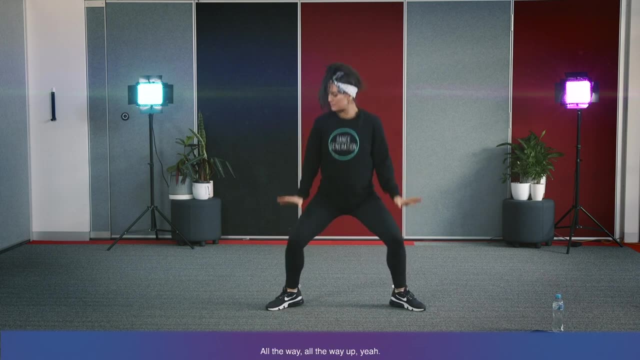 Let's do some shoulders Right up Down Good, Warming up all of our joints All the way up, All the way up Down And single Up And up Double time. We go two at a time. 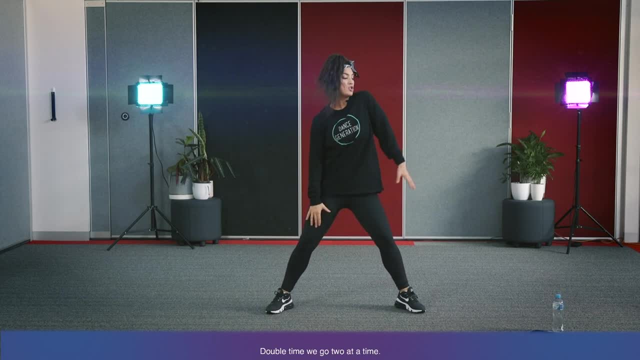 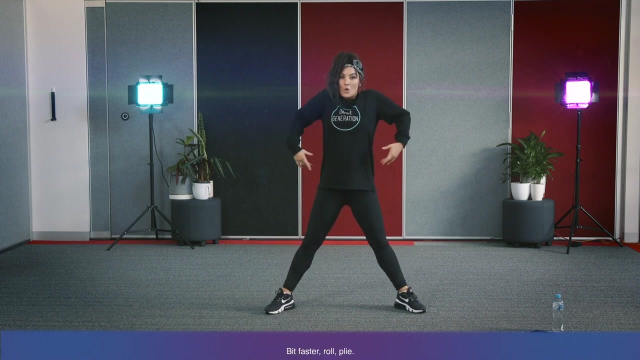 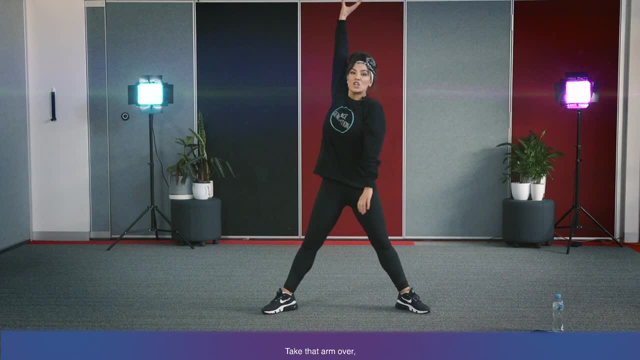 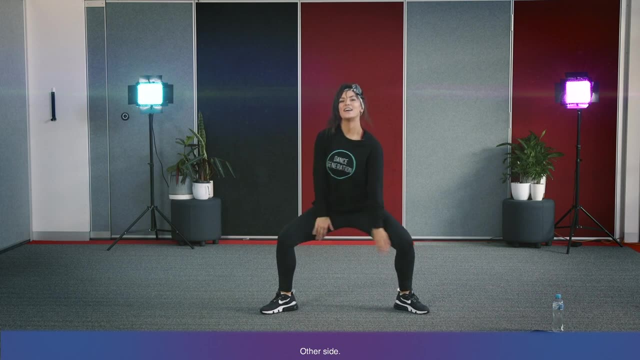 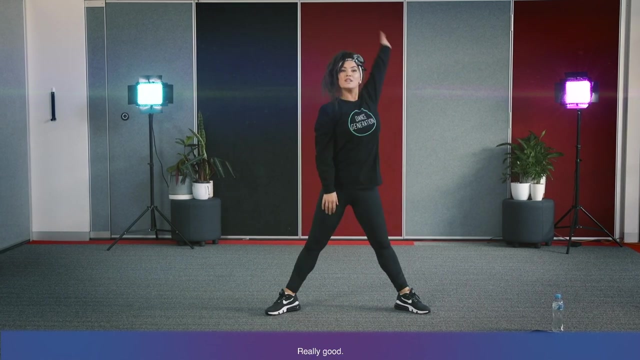 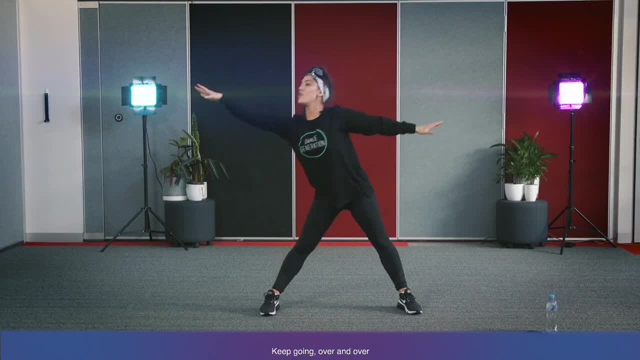 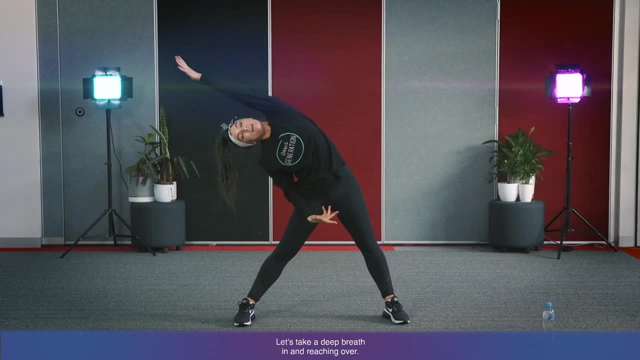 And my legs are nice and straight And I'm just reaching over. Keep going Over And over And over. Alright, let's take a deep breath in and, reaching over and hold that. You should feel a stretch in the side of our body. 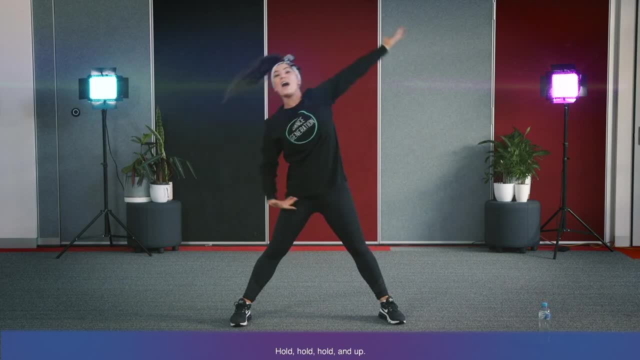 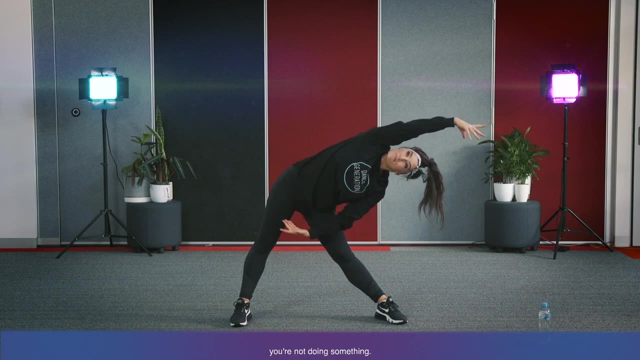 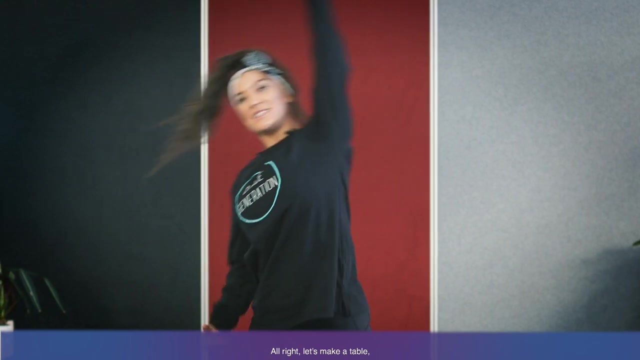 Hold, Hold, Hold And up and up other side and over breathe. You can feel the stretch here you're not doing something- And over again for the second time. hold it there. All right, let's make a table reaching out. 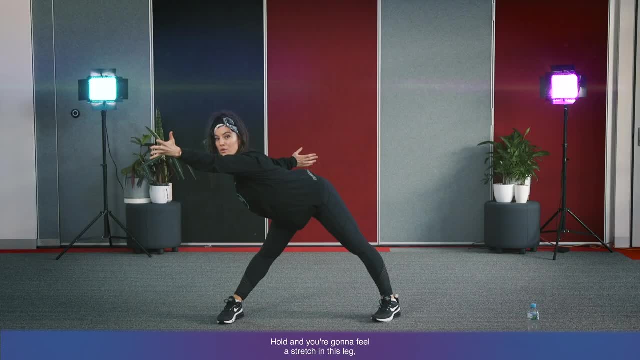 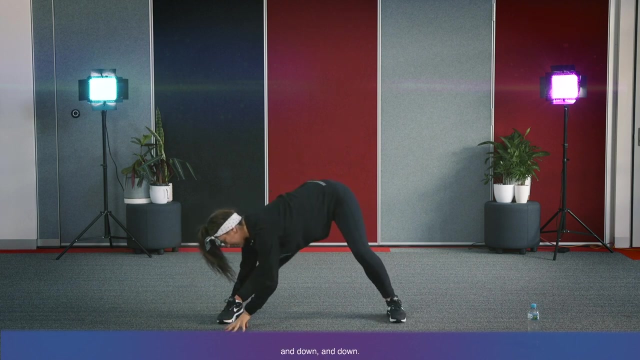 Try to get this part of your back really flat. hold And you're gonna feel a stretch in this leg. Let's go down to this leg. See if you can get your stomach onto your leg, Breathe and hold. Let's bend our back leg and down and down. 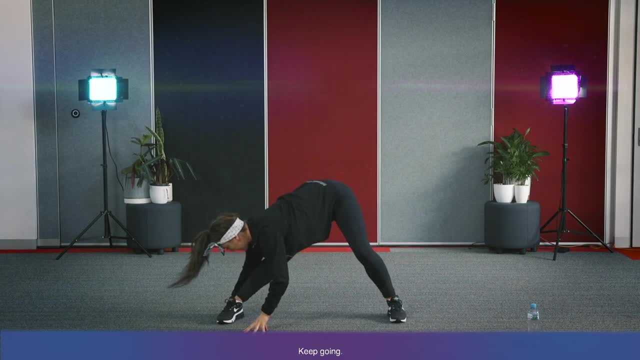 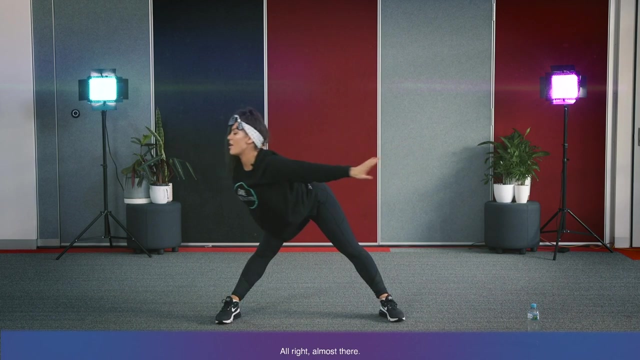 All about warming up all of our muscles. Keep going good, Four more and one, two, three, four. Let's go back to our flat back, hold And going around and around- all right, almost there, Reaching up and over, breathe and hold. 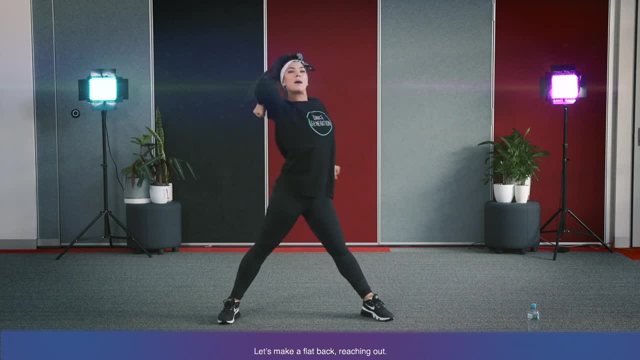 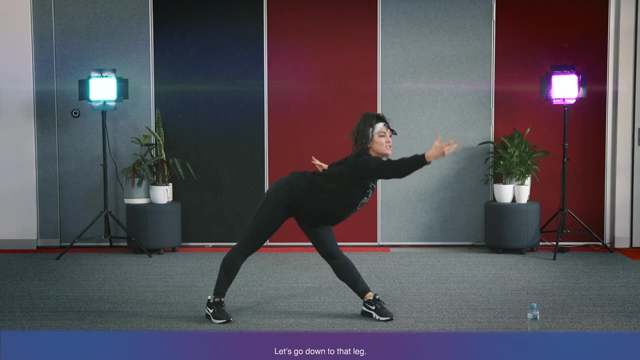 I can feel a stretch in the back. I can feel the stretch inside of my stomach here. Let's make a flat back reaching out. Good try to get this part of our back really flat. Let's go down to that leg. 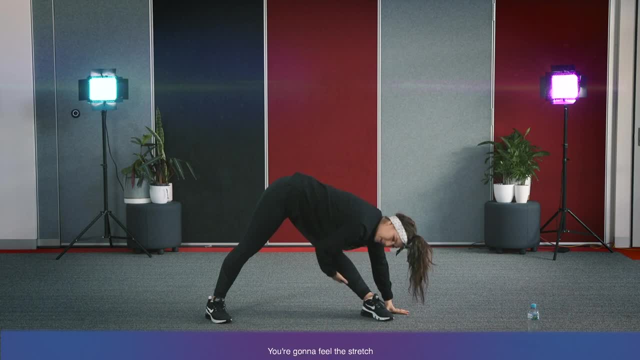 See if you can get your stomach on this leg. You're gonna feel the stretch in this leg here. Let's bend this leg and down, down. I hope you guys are starting to warm up Almost there. four more, all right. 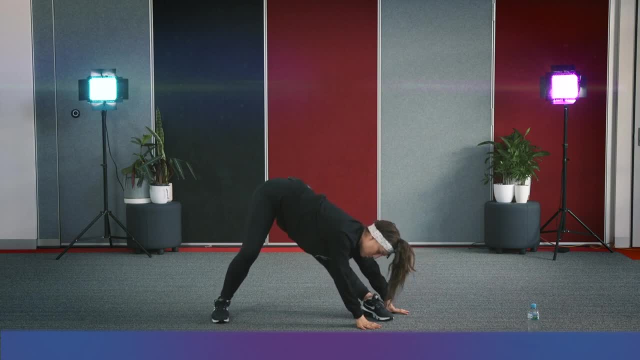 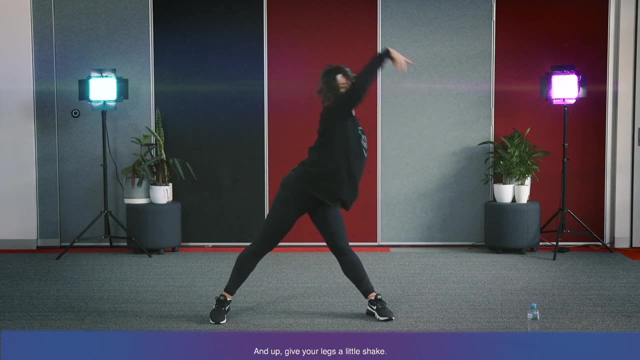 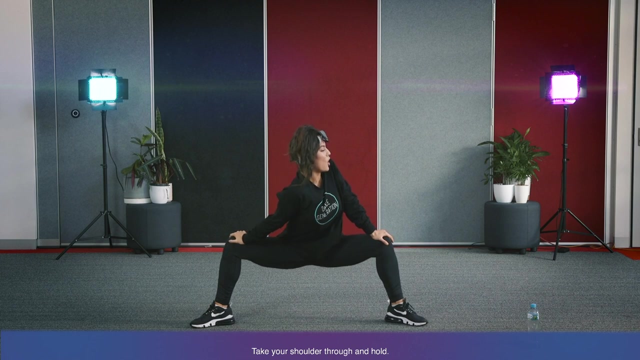 One, two, three, four. Back to flat back and around and around and up. Give your legs a little shake, Press your knees out to the side, Take your shoulder through and hold, Feel that stretch Other side and through breathing, other side again. 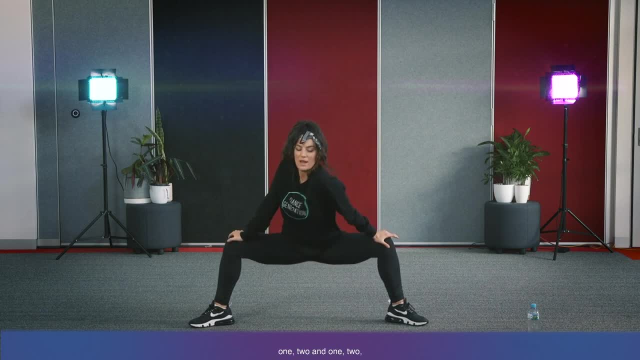 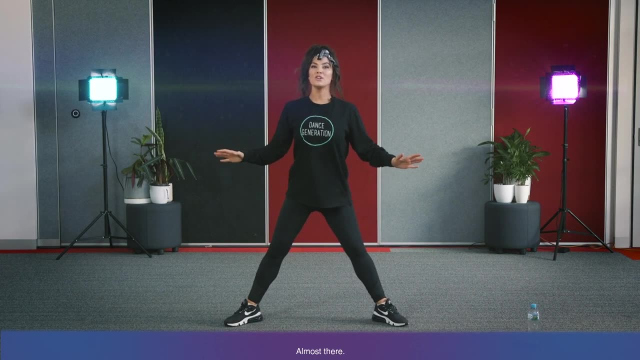 One, two, change one, two and one, two, and one, two, Two, one, two. Give your legs a little shake. Almost there, You can go back to here. or if you want a deeper stretch, you can go elbows to knees. 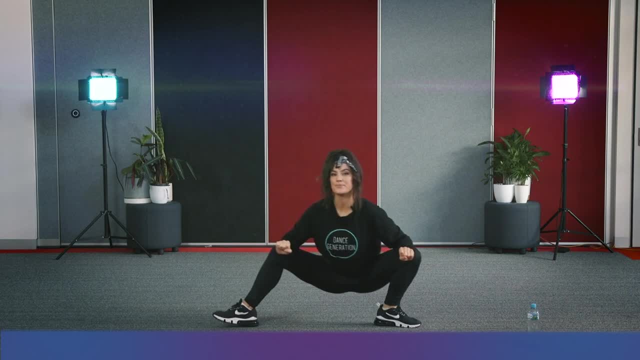 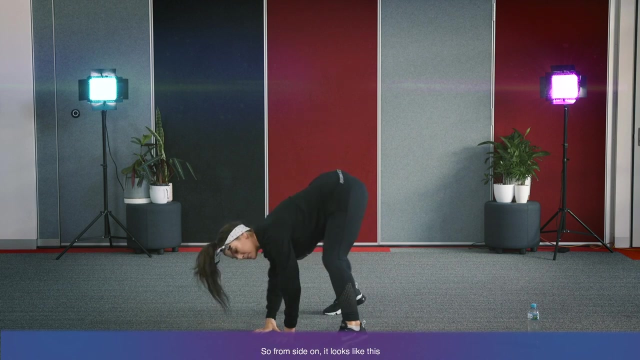 Rocking side to side, Good guys, Stretching our legs Almost there. And now we stretch our legs and we're hanging over. So from side on it looks like this And I'm stretching out my back: One, two, three, four. 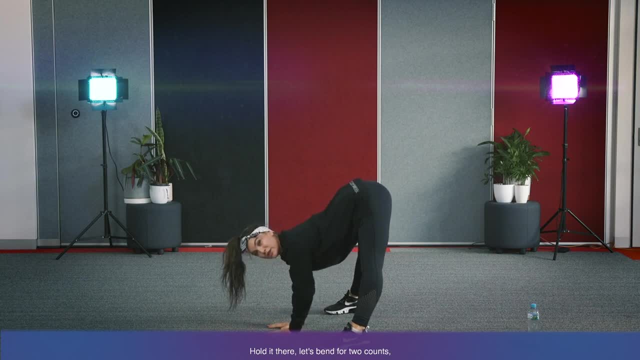 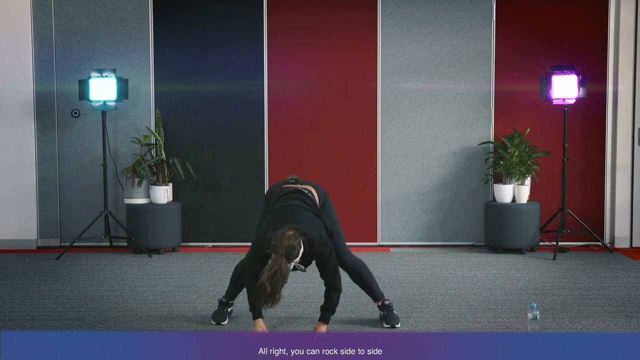 Stretching out the back of my legs. Hold it there. Let's bend for two counts. We go: bend two and stretch And bend, and stretch, And bend and stretch. All right, You can rock side to side and make a cradle or a carriage and just let your back hang. 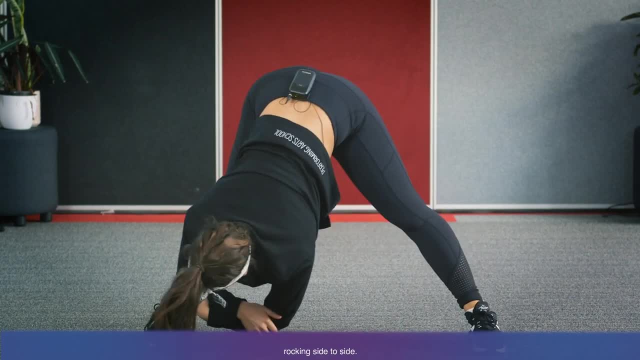 Rocking side to side- Really good. You're going to feel it in the back side and in your back, So you're going to stretch. just suck in your back. You're going to feel it in the back, So you're going to bend your foot. 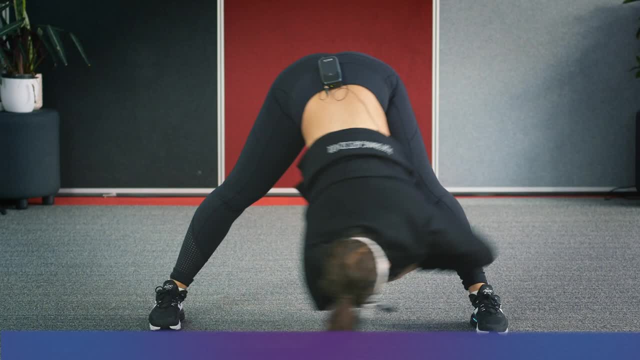 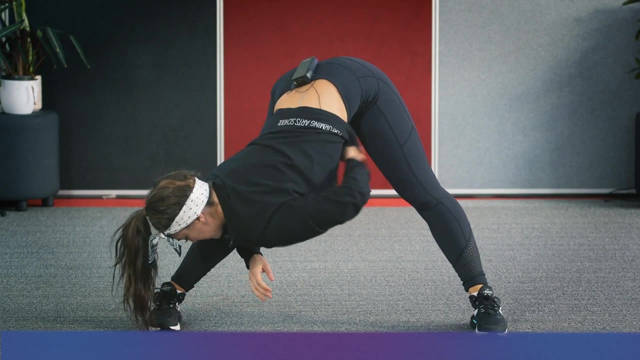 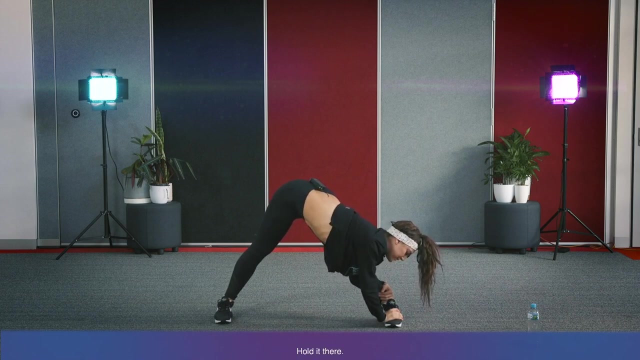 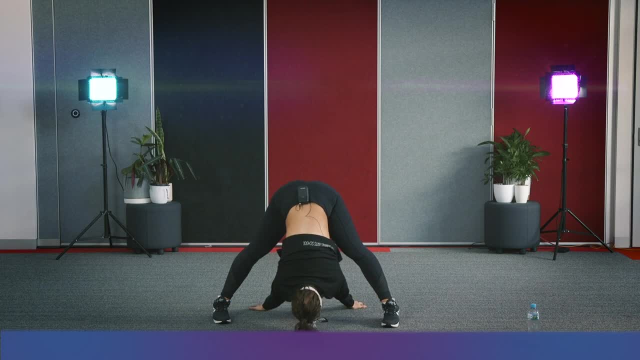 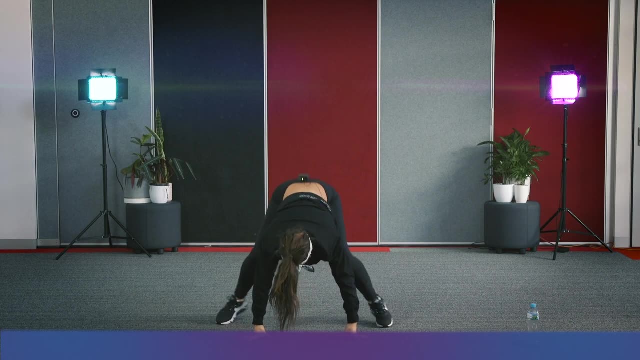 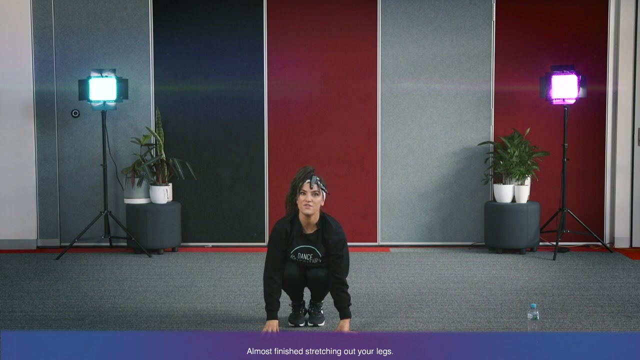 feel that stretch. hold it there breathing. hold it there really good. let's walk our feet in and bring our heads up. hold it there. almost finished stretching out your legs and hanging back over. feel that stretch in the back of your legs and down. give your head a little rest last time and over and slowly rolling up. 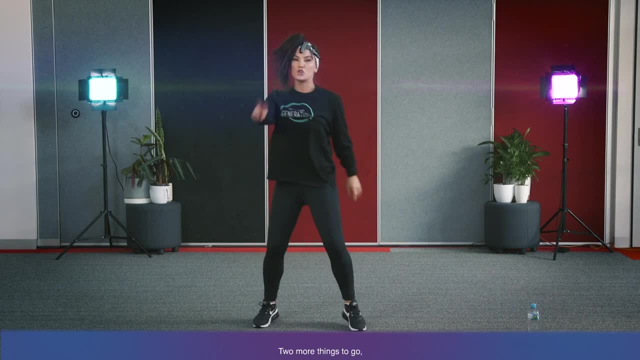 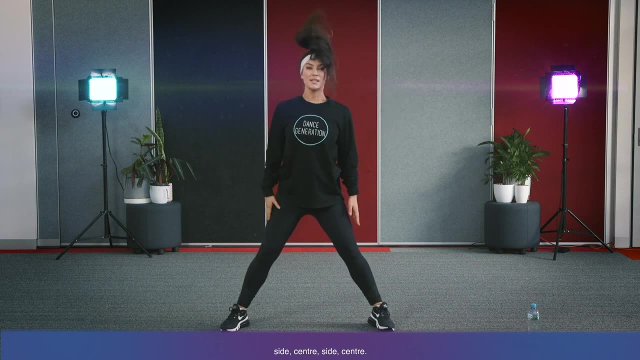 really good, give your legs a little shake. two more things to go. let's stretch our neck side, center, side, center, side, center. and to this side, side, side and side, really good. and forward and forward, lovely. let's do a half circle down there, other way to the back and round. 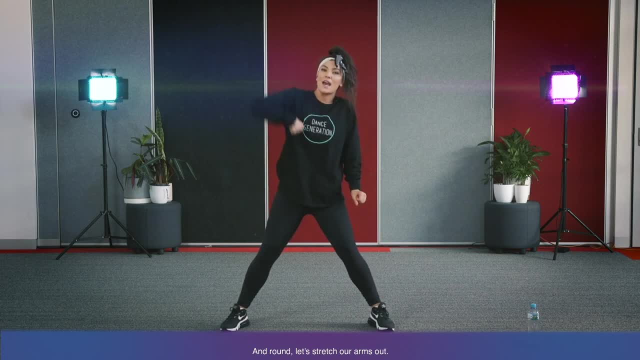 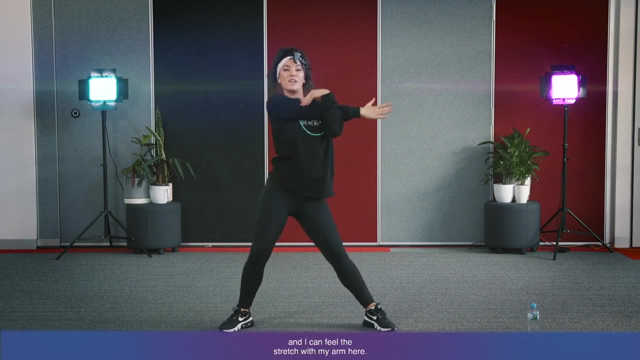 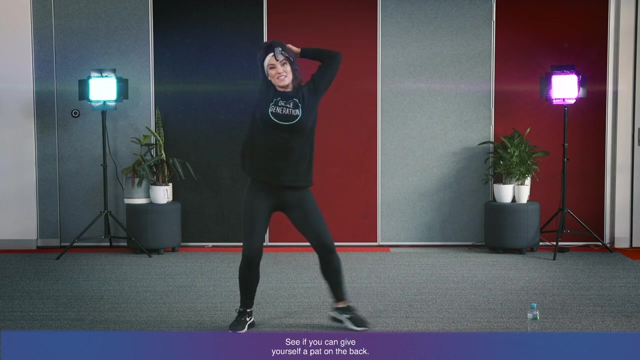 and around. let's stretch our arms out up, take it across your body and take that arm under. i'm gonna pull this arm in and i can feel the stretch in my arm here. good, all right, hold it there. let's take that same arm up and over. see if you can give yourself a pat on the back. 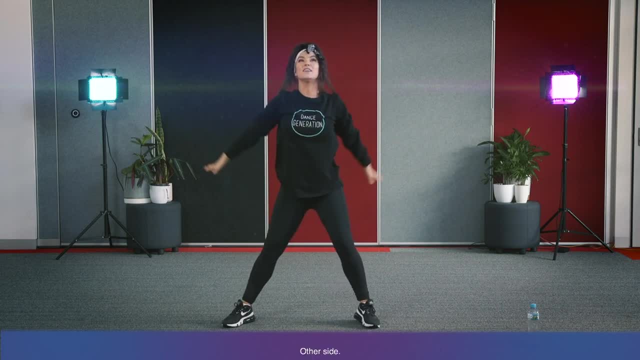 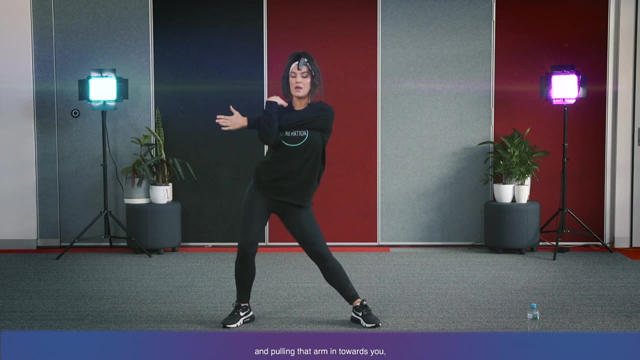 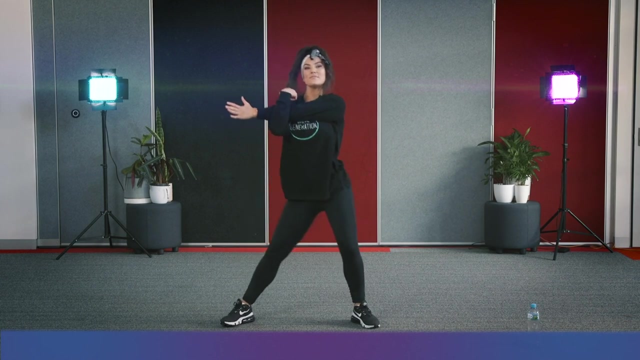 feel that stretch and pull it across. give yourself a pat on the back if you can hold it there. feel that stretch and pull that arm in towards you. i can feel a stretch in this part of my arm. good, keep going and take it up and over, pull it across. give yourself a pat on the back if you can. 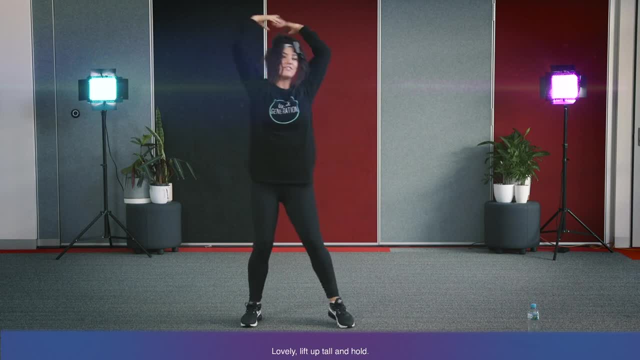 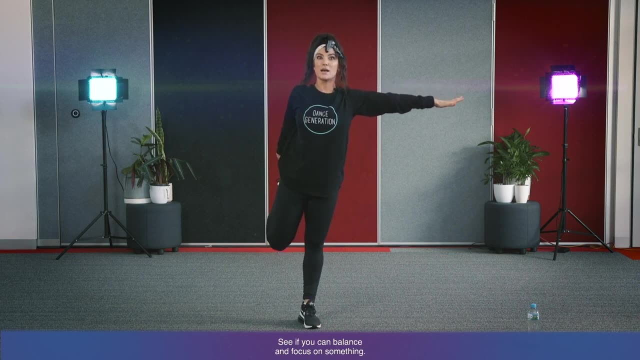 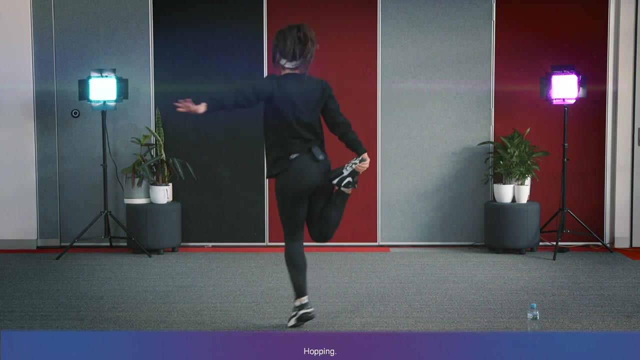 hold it there, feel that stretch lovely. lift up tall and hold, see if you can balance and focus on something. and do two circles around yourself popping, and see if you can balance now really good. other side, lifting up tall, imagine a spring pulling your head and making you grow two circles around yourself. 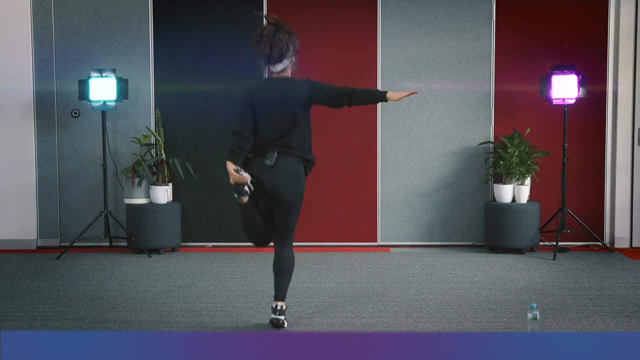 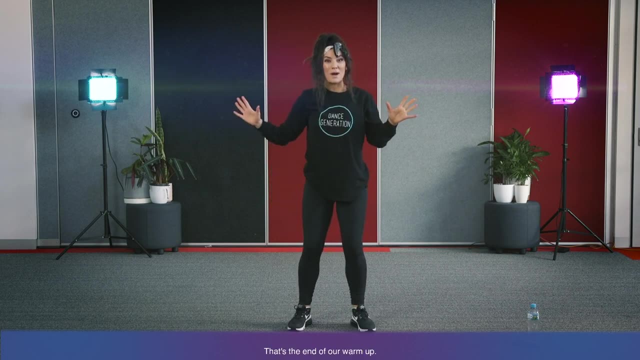 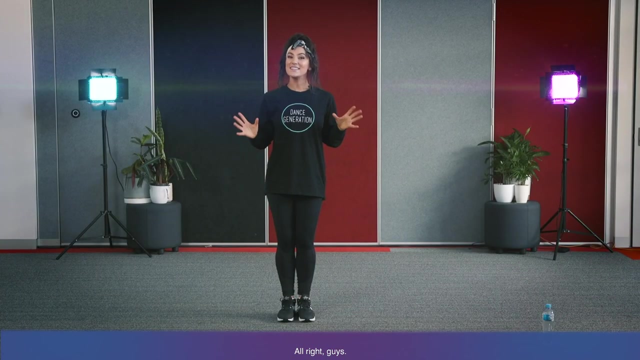 doing three circles around yourself by kolina. keep going, see if you can balance. wonderful, that's the end of our warm-up. have a little drink of water and let's start learning a routine together. i'll see you guys in one second. all right, guys, let's get started. let's. 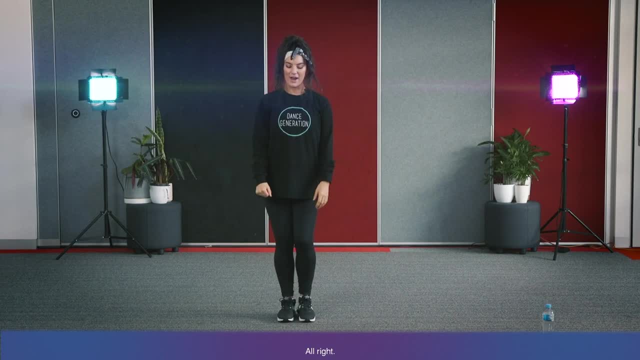 start learning our hip hop routine today. all you have to do is mirror exactly what we do, because we've flipped this video for you. all right, bend our knees. we want your feet back up and forth with your hands out around. youkanuu really got to bend our knees for hip hop. It's going to make it feel more hip hop All. 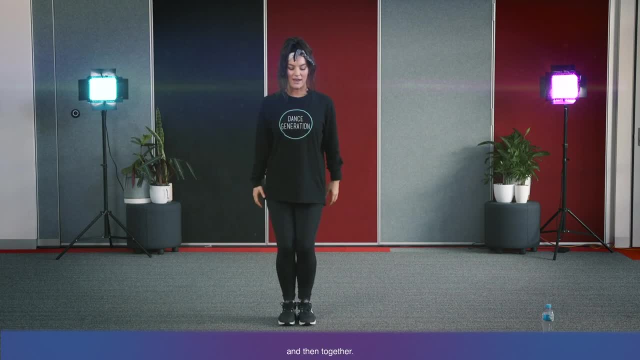 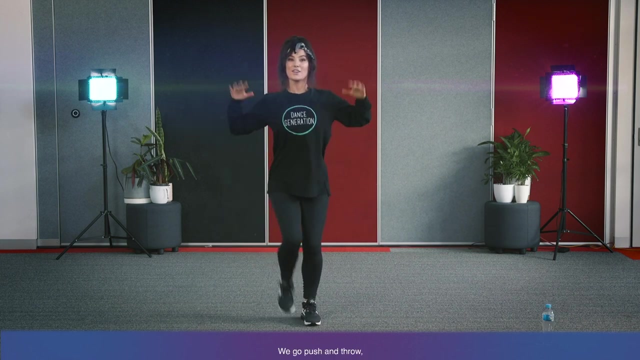 right, All we're going to do is step out to the side and then together, Side and then together. I'm going to add in a little push with my hands and I'm going to throw my arms away. I'm going to push, throw it away. We do two of those: We go push and throw, push. 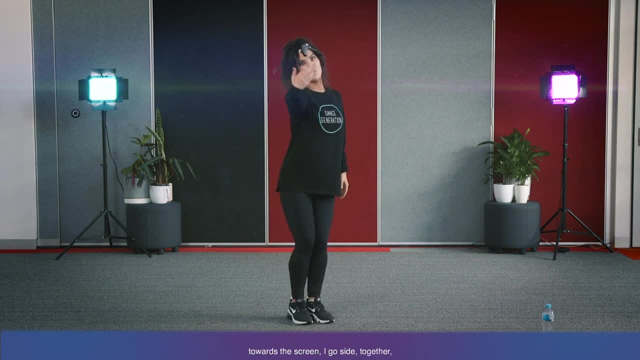 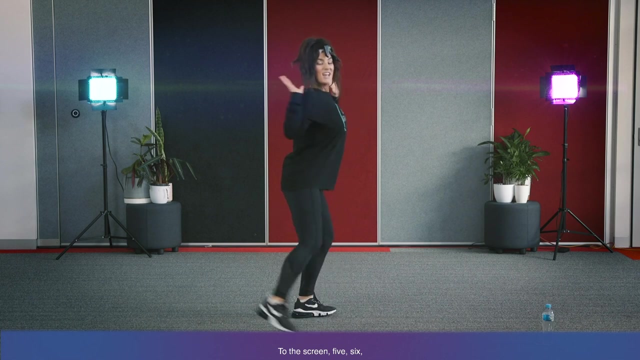 and throw. I do the same step towards the screen. I go side together, side together. We have four of those, Let's go. We go one, two, three, four to the screen, five, six, push seven, eight. One more time a little bit faster. We go, push one together, two. 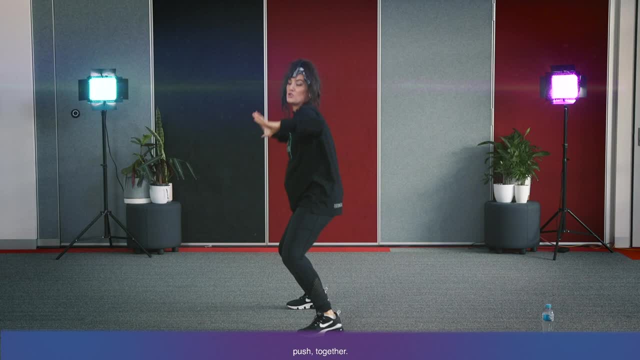 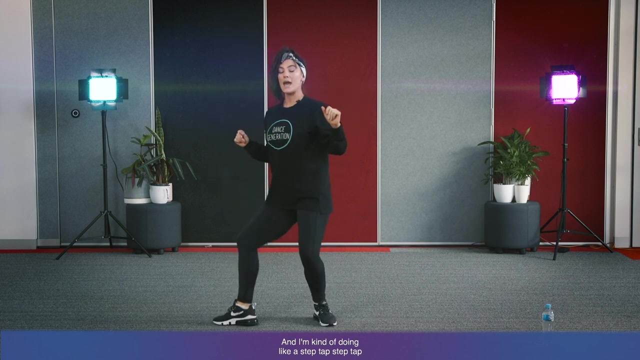 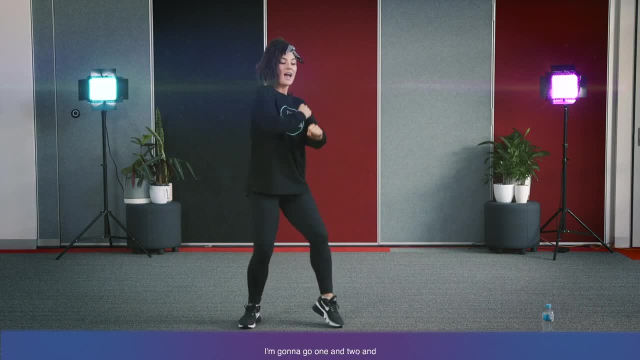 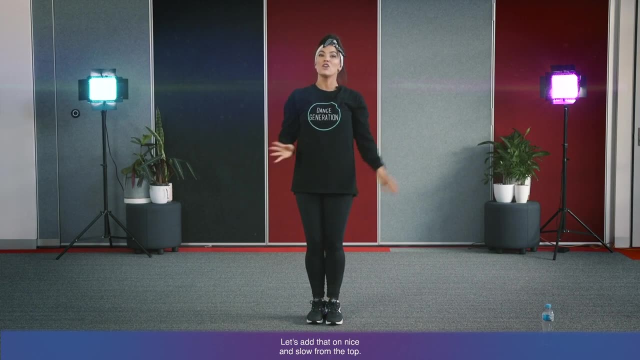 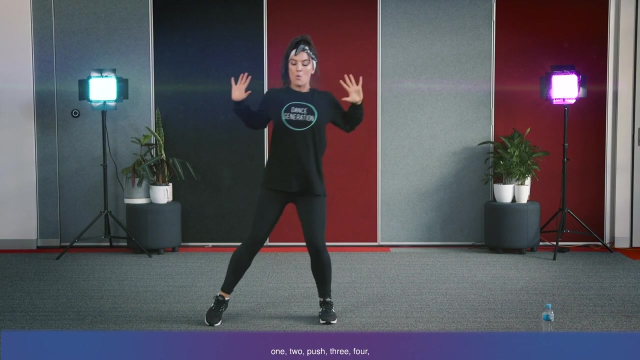 going to do four of those. I'm going to go one and two and three and four, and Let's add that on nice and slow From the top. Whenever I do this, I mean from the top, We go with our push. step One. 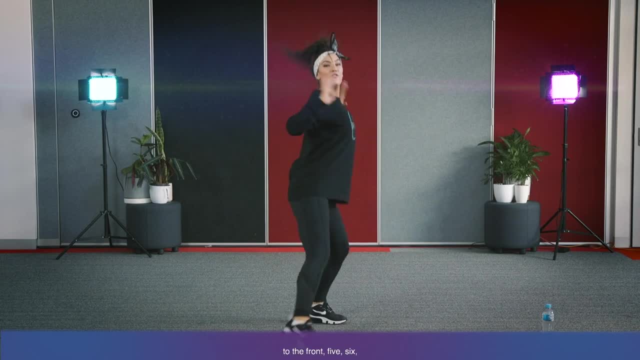 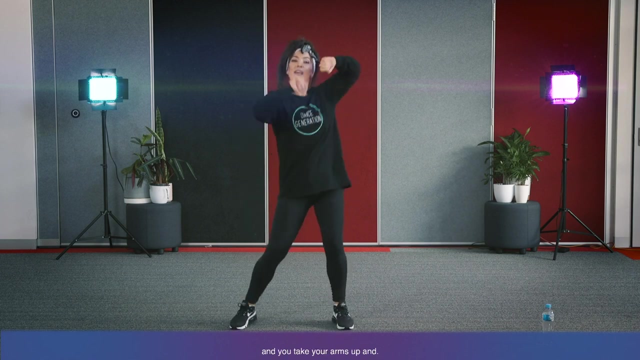 two push three, four to the front, five, six, seven to the side. We go one and two and three and four, and So that to the music will be like groove and groove and you take your arms up and Yep. after there I'm going to do four walks. 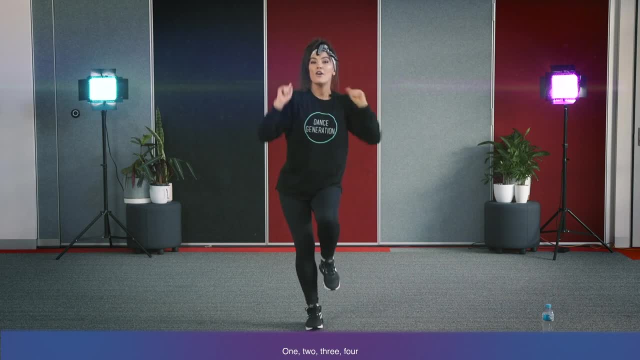 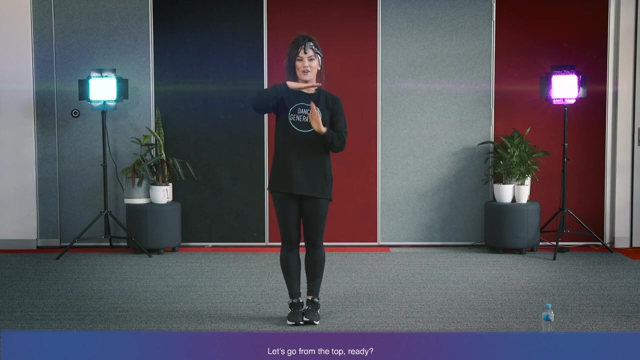 I'm going to go one, two, three, four, And my arms are just going up and down, and up and down. we're pointing: Yep, it's pretty groovy. just four walks. I'm getting puffed. Let's go. from the top Ready to the side we go, and you guys can give it as much as. 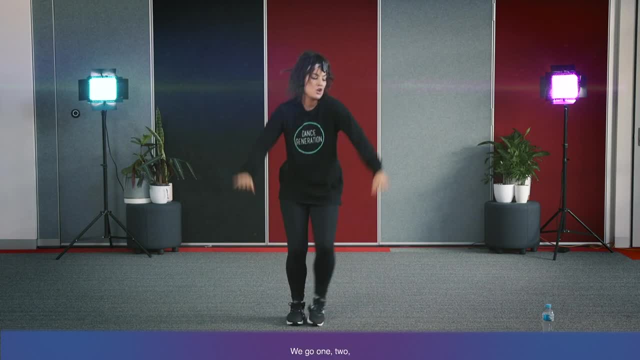 you want with this. That's up to you. We go one, two, three, four. I'm going to, you're going to walk. The trick is, you're going to have my arms were like up, down, up and. down, up, up, down, Up and down. That's up to you and you just need to get it on top of it. casa acerca y una récupolo. One, two, three and up You come off. I'm going to lift up, I jump out of my seat and 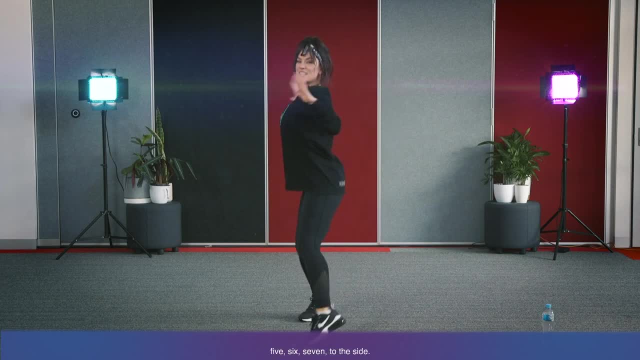 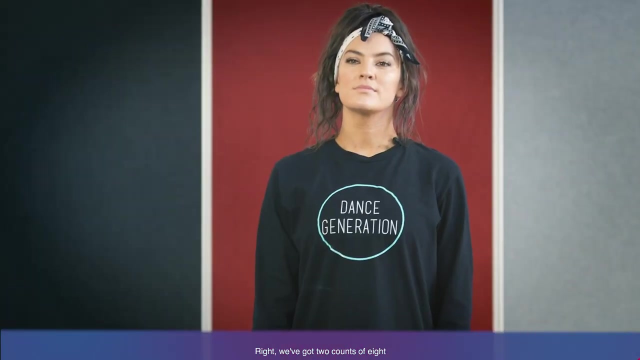 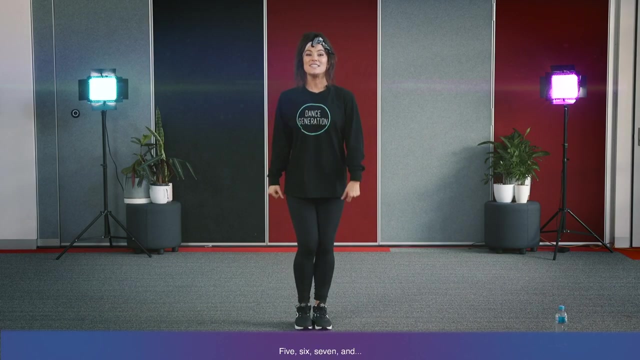 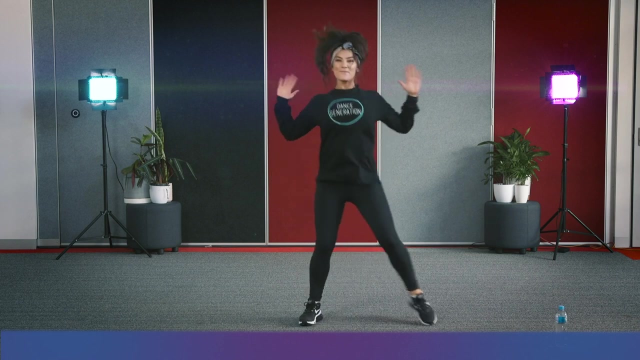 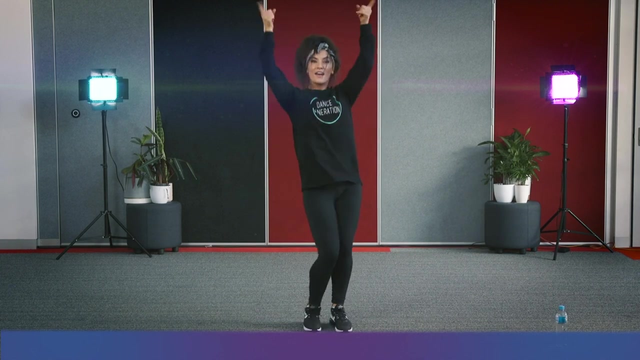 four to the front, five, six, seven to the side, one and two. and party arms: four steps up and down and up and down. let's do that much to music, okay. to the side: four walks and up. let's do it again ready. okay, don't worry if you didn't get it, you're just learning together. let's go five, six, seven and push to the front. to the side: four walks and up. 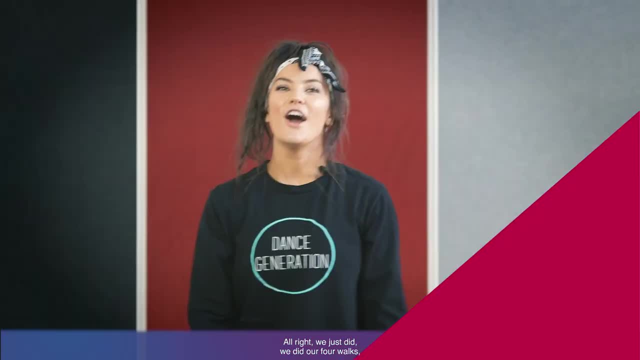 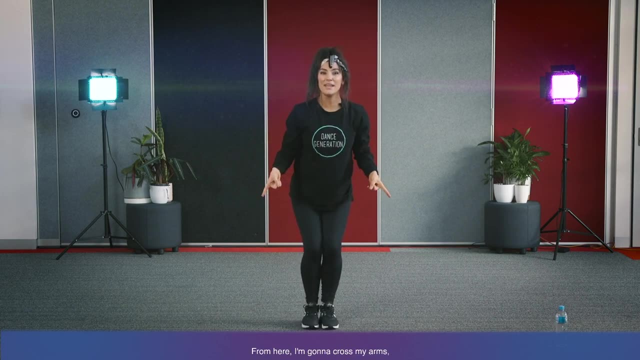 all right, let's start learning the next part. all right, we just did. we did our four walks. we went up and down and up and down. from here i'm going to cross my arms, touch my shoulders and i'm going to reach out nice and strong and when i reach out from side, on it. 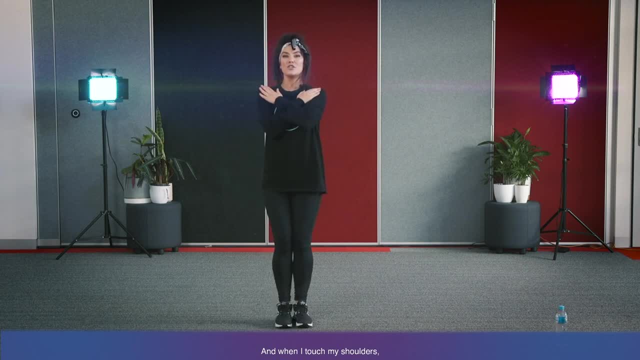 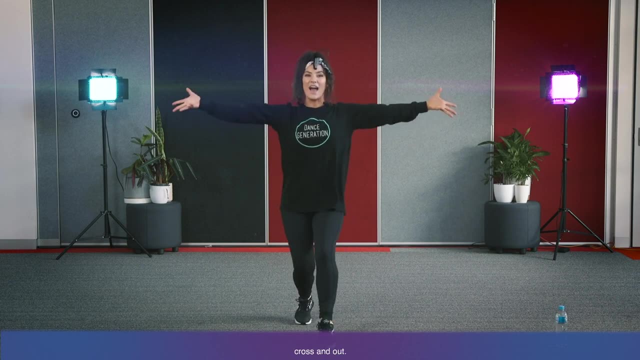 looks like this: my legs come out when i touch my shoulders, my feet come back, and we're going to do two of those. we go cross and out, cross and out. all right, let's add it on. from the walks i went up and down and up and down. 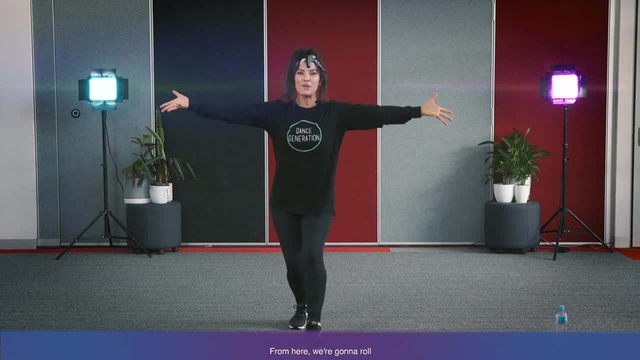 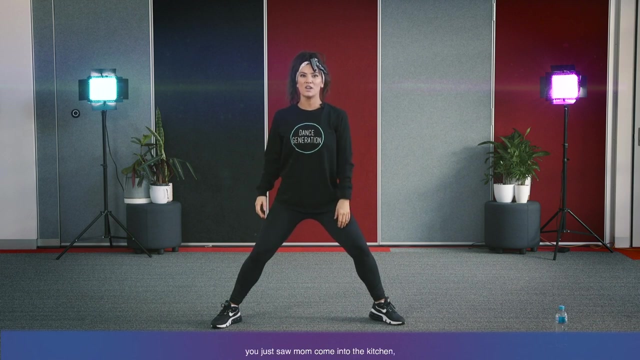 cross out, cross out from here. we're going to roll and jump at the same time. I'm gonna go one, two, jump my feet out from there. I go roll one, two. I'm gonna go look, look. so you just saw someone. you just saw mum come into the kitchen, or? 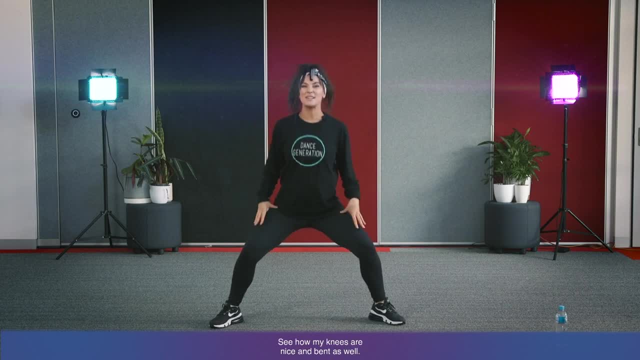 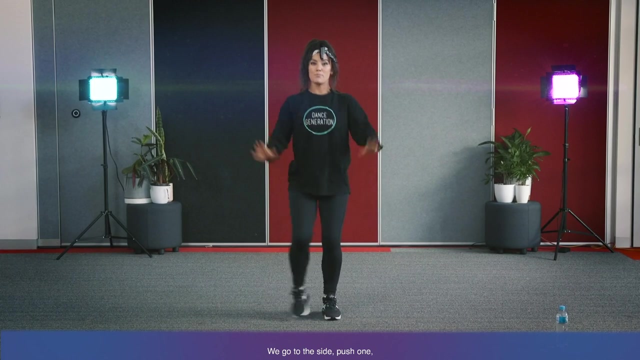 someone's watching you dancing. see how my knees are nice and bent as well. I went cross out, cross out. I roll one, two, three, four. cool, let's go from the top without music. we go to the side, push one, two, three, four to the front, five bend. 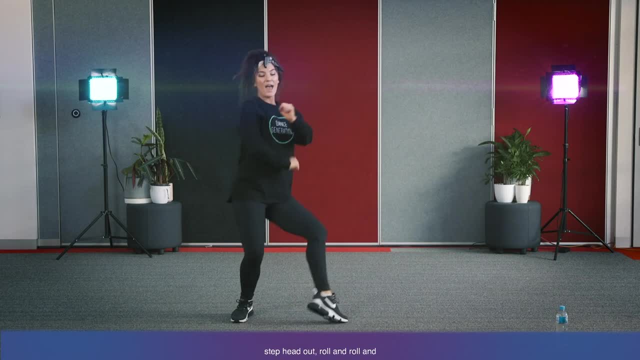 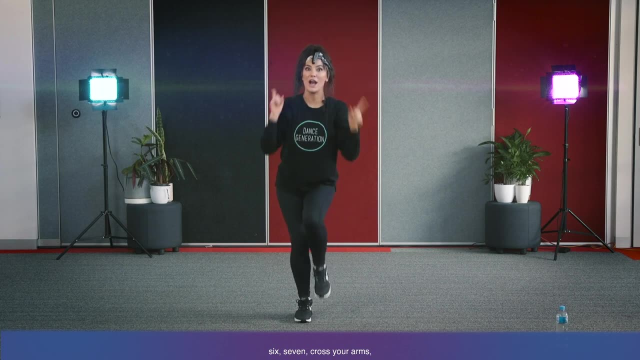 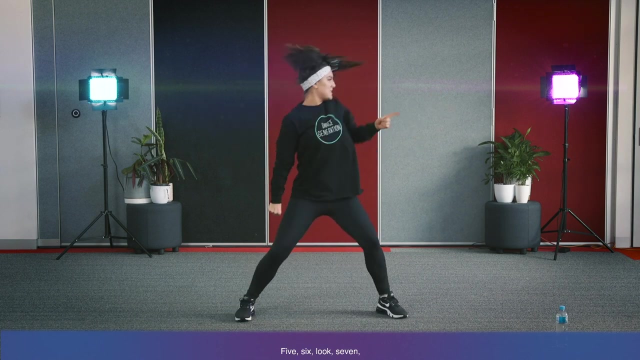 your knees and seven, step it out, roll and roll, and three and four, we're walking. five, six, seven cross your arms. next step: oh, 1,, 2,, 3,, 4, we roll, 5,, 6,, look, 7,, look 8.. 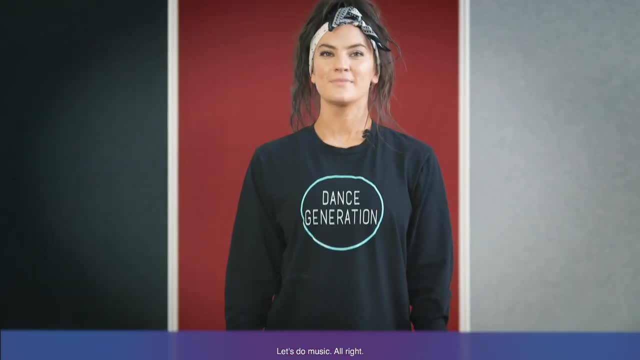 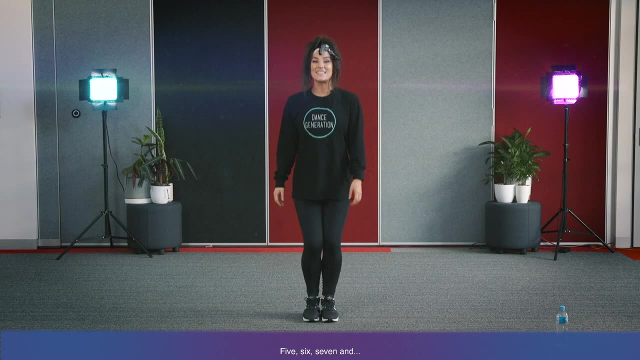 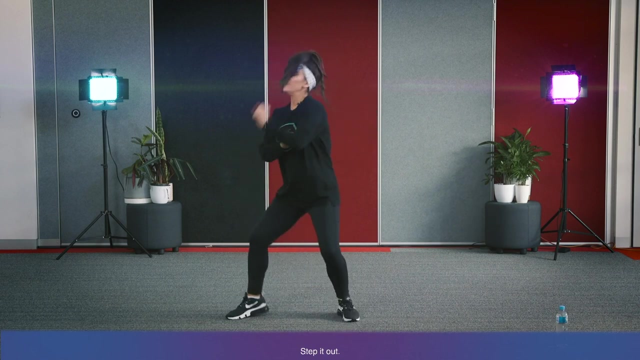 Cool, Let's do music. Alright, Just relax, We're going to have some fun. Let's go 5,, 6,, 7 and push To the front, To the side, Step it out, New step And let's roll. 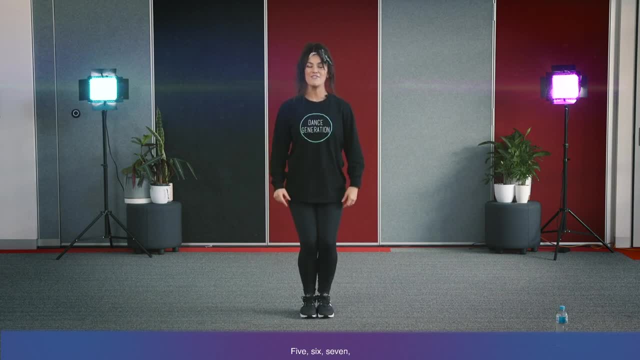 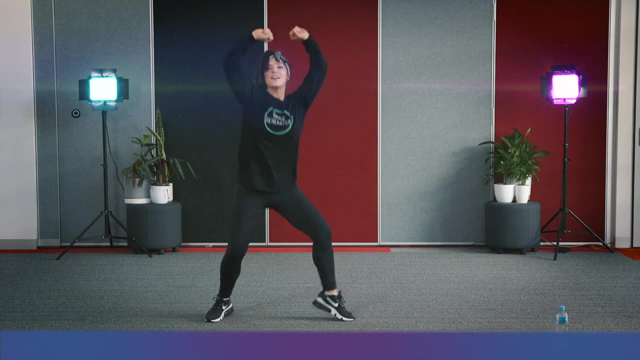 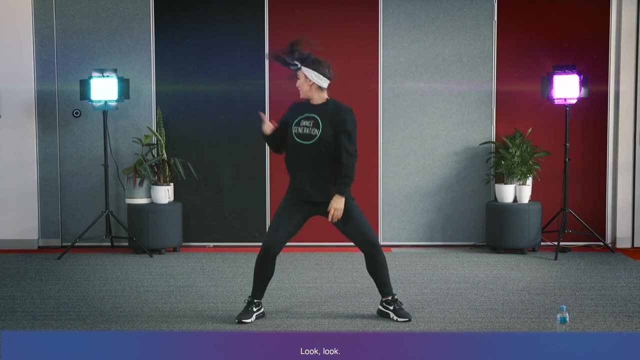 One more Ready: 5,, 6,, 7,. push it 1, to the front, Step it out And walk. We'll cross And up. Look, look, Alright guys, let's add on, Let's go. We just did cross and out. 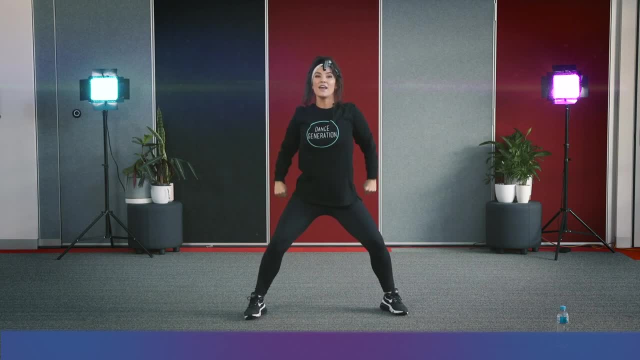 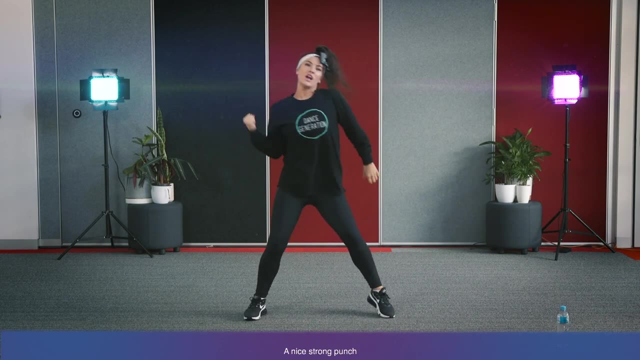 Cross and out. We rolled here and look, look, From here this hand. we're going to come back to the front and I'm going to go hit Nice strong punch And I'm going to put my body into it as well. 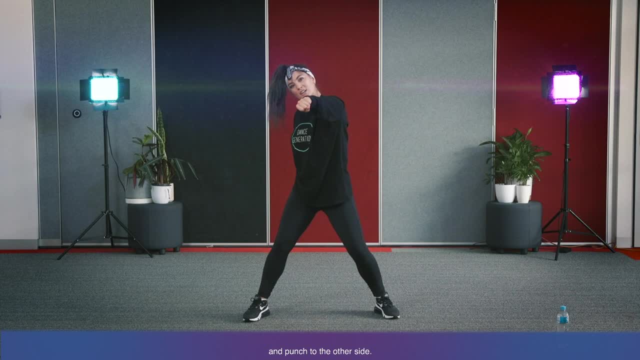 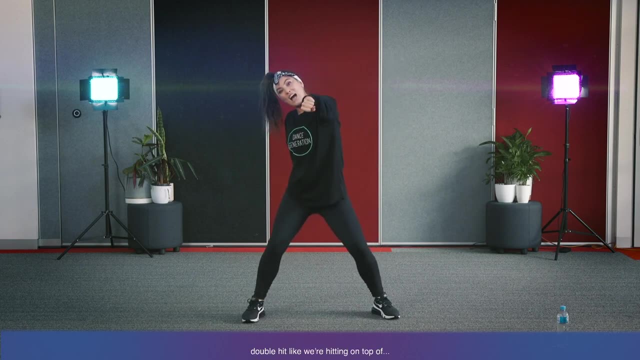 I'm going to go punch and punch to the other side, Just two punches. I went look, look, I go hit and hit, Double hit, like we're hitting on top of I'm not sure You can imagine something. 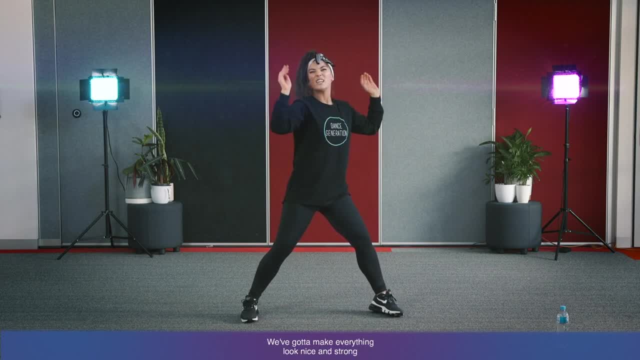 But you've got to let your arms stop there so your arms aren't floppy. Yeah, we've got to make everything look nice and strong, And I'm going to bend my knees, And if you want to put some chest into it, that's fine as well. 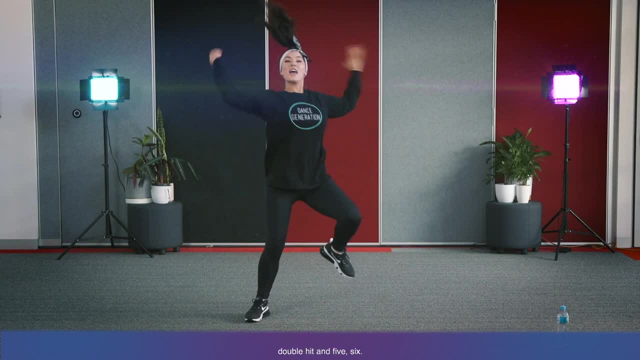 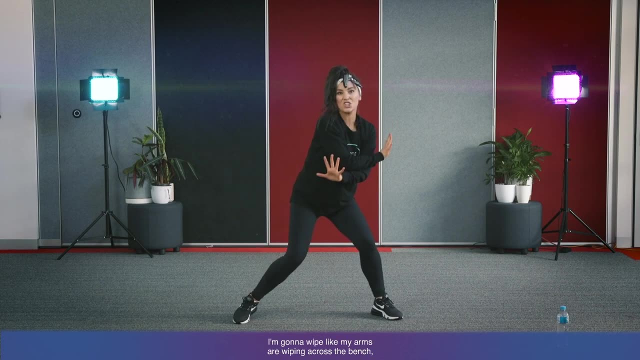 I went: hit, hit, double hit And 5,, 6,- next part, moving on, I'm going to wipe like my arms are wiping across the bench, Wipe, jump. Okay, Let's take it back from the cross. 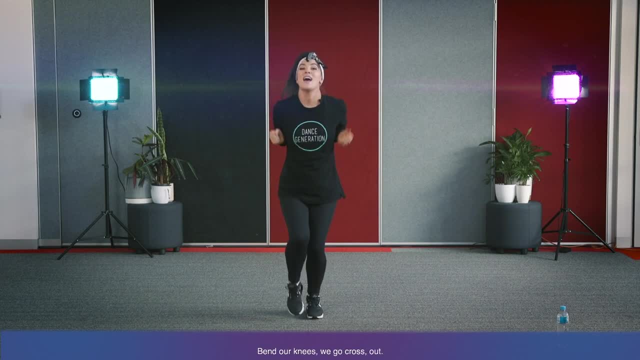 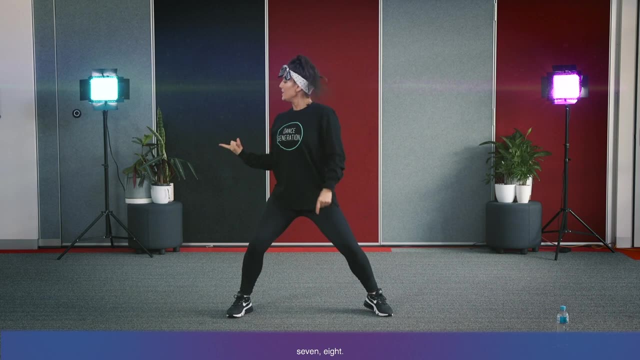 Feet together, Bend down knees. We go Cross out, Cross out. We roll 5,, 6,, 7, 8.. I punch it 1,, 2,, 3,, 4. Double hit. 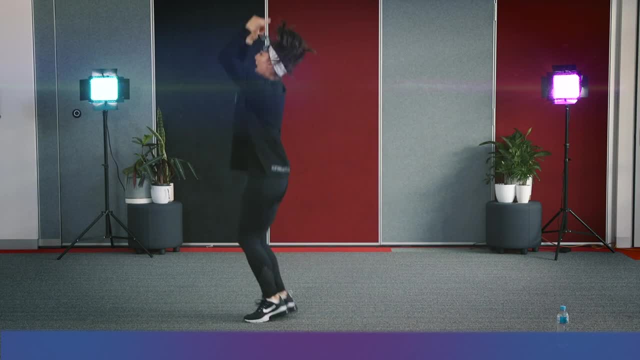 5, 6, wipe 7, 8.. Let's keep going. I think you guys can keep going from here. From here, I'm just going to groove for two counts and I'm going to roll. I'm going to do two steps. 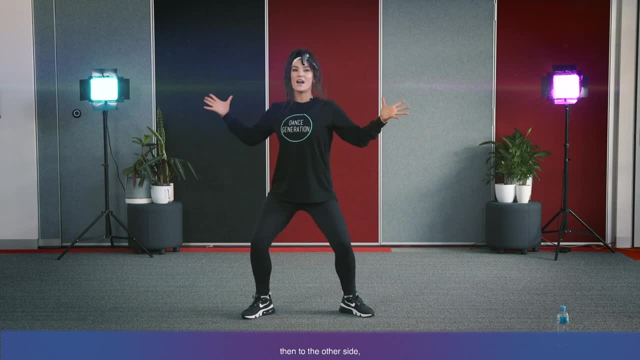 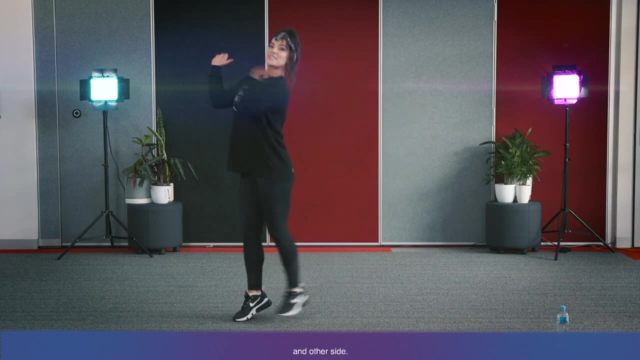 I'm going to go roll and roll, Then to the other side, Clap Same thing. this way, I go roll and roll and other side. So we get to do that twice. Okay, Let's take it back from here again. 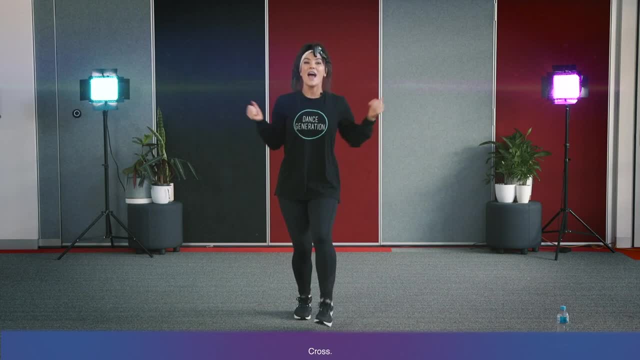 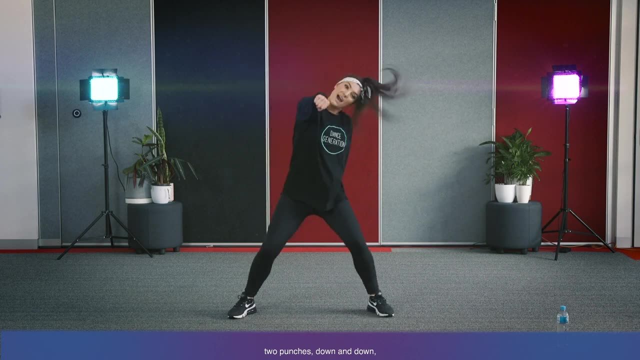 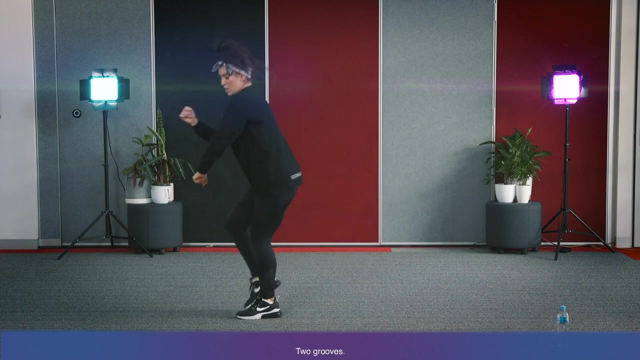 Cross out, Cross out, I jump. 5, 6.. I look: 7, 8.. Two punches down and down, double hit and hit, hit and wipe, Little Little Little jump. Two grooves, two steps to the other side, two steps and I'm just kind of over. 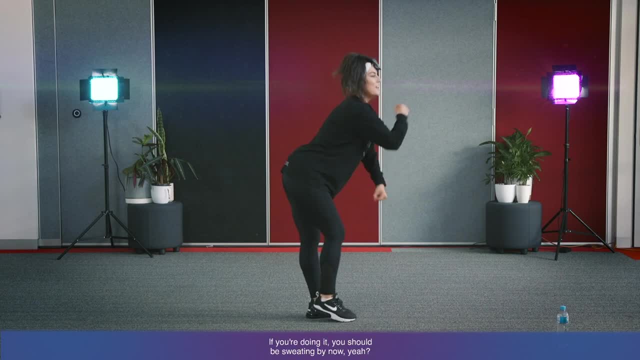 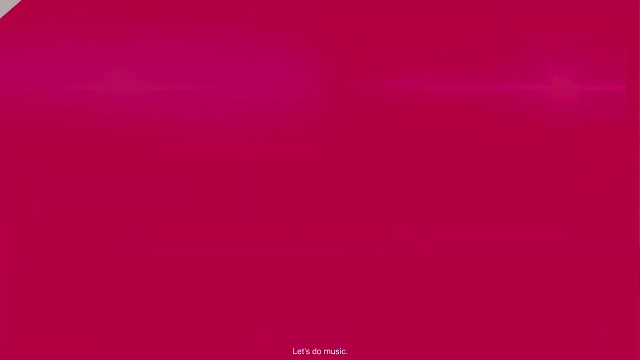 Quite a workout this guys. if you're doing it, should be sweating by now. yes, Roll it to the other side. Okay, Do you want to try music? Let's do music. We're going to step out to the side. 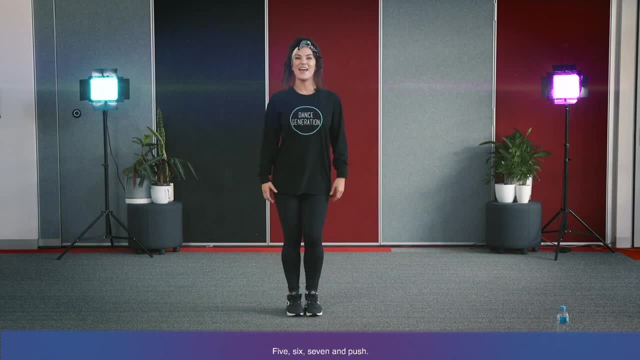 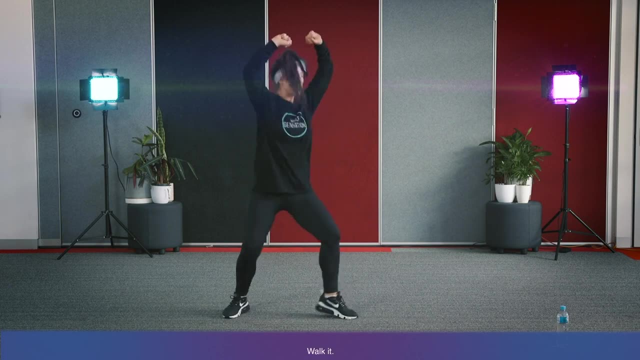 Let's go flat out: 5,, 6,, 7, 8.. Push to the front, Step it out, Walk it And crawl, Roll it, Then punch and punch and punch, Double hit. That's good. How did you guys go? 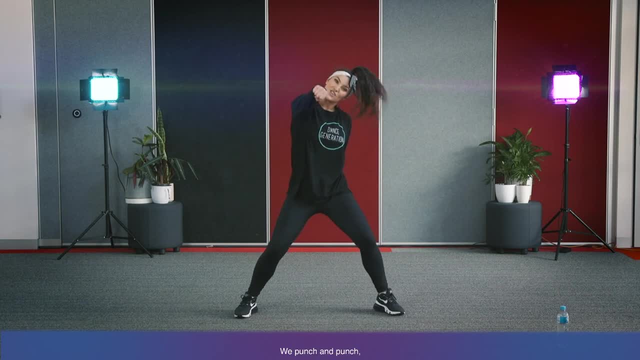 Let's go again: 5,, 6,, 7 and 1., 2., 3., 4. 5,, 6,, 7,, 8. Push to the front, Step it out, Walk it. 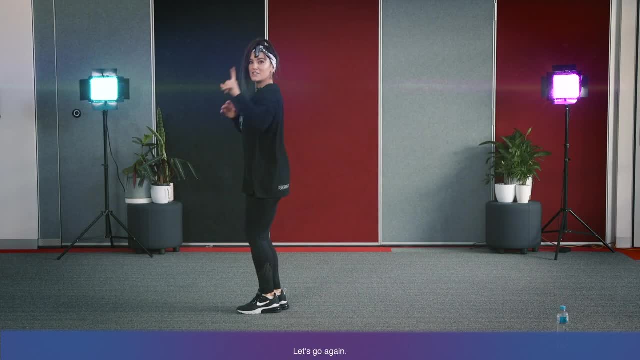 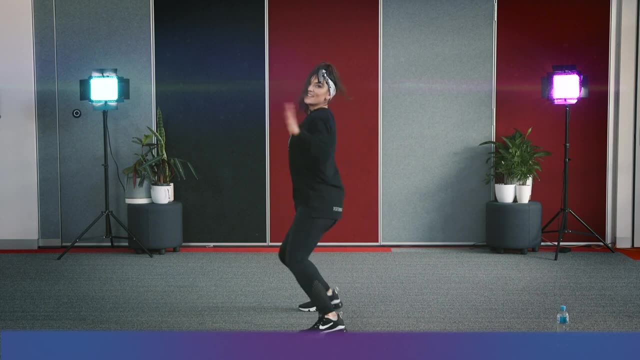 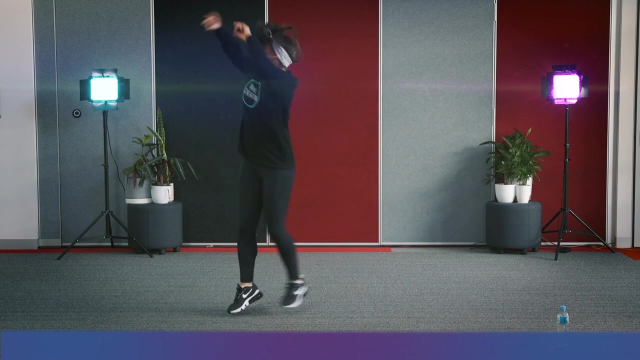 And crawl, Roll 2., 3., 2. And punch Double hit. That's good. How did you guys go Kick back, kick back, walk it, kick back and up and kick it and groove to the other? 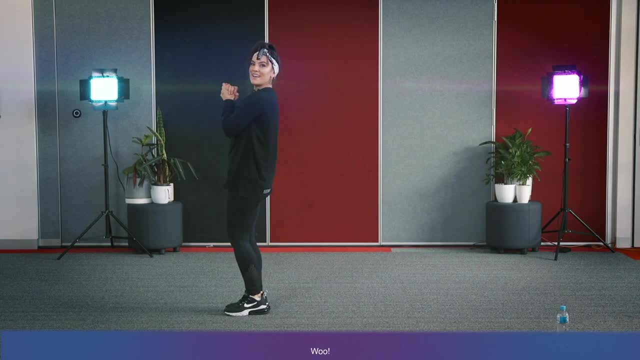 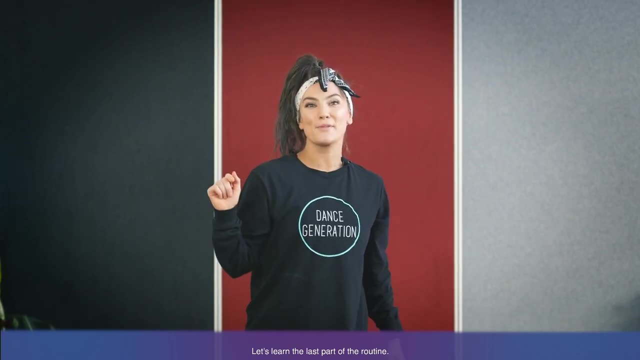 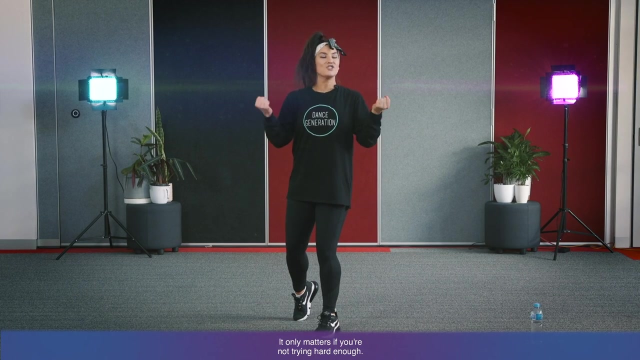 side, Get a quick drink. Alright, I'm puffed because I've been talking so much. Let's learn the last part of the routine. okay, And it doesn't matter if you're not getting it right, it only matters if you're not like. 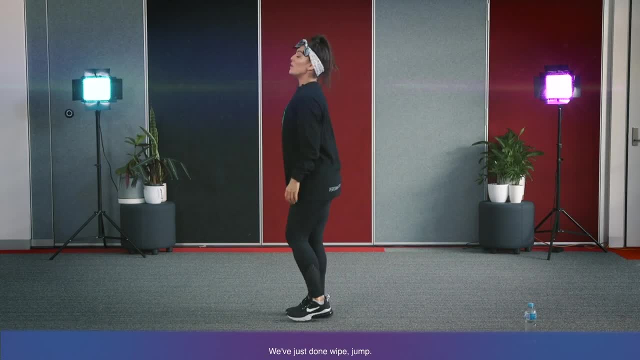 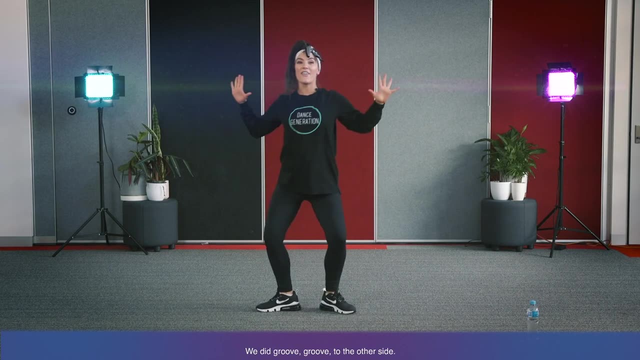 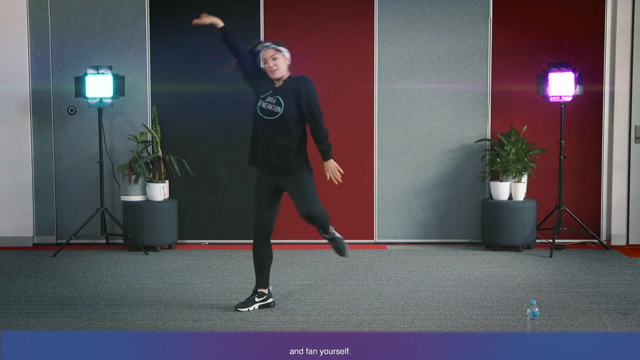 trying hard enough, Just give it a go. It's all about having fun. We've just done wipe jump. We did groove groove to the other side. Groove, groove to the other side. You're going to step out and fan yourself. 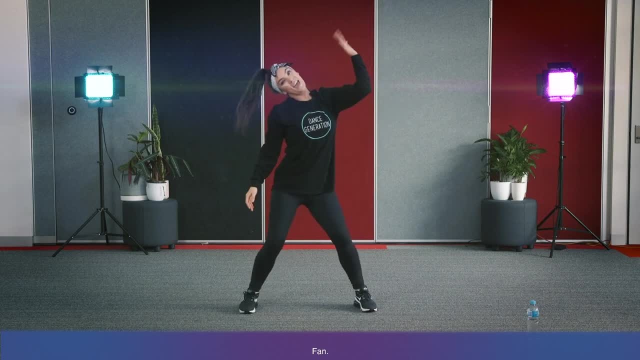 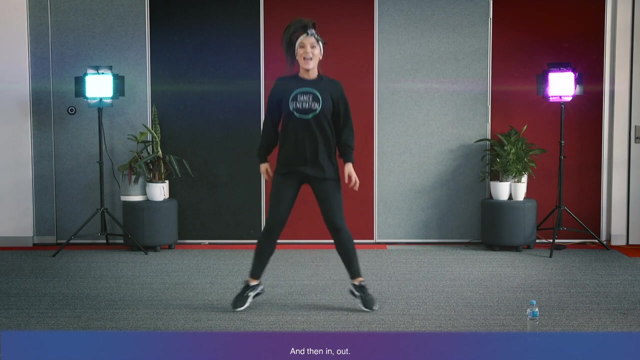 Oops, I'm all wobbly Fan fan. This hand, This hand here is going to go knee, knee, jump in out. okay, I've got two fans, I've got two knees And then in out. 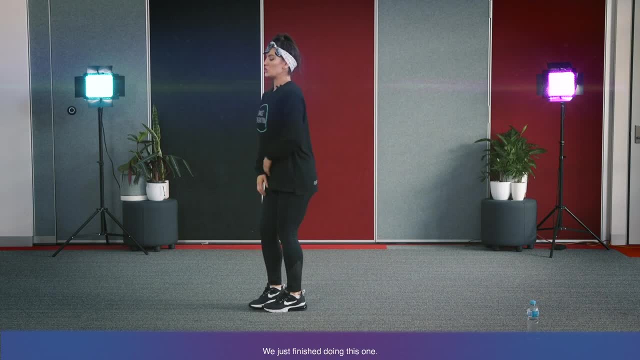 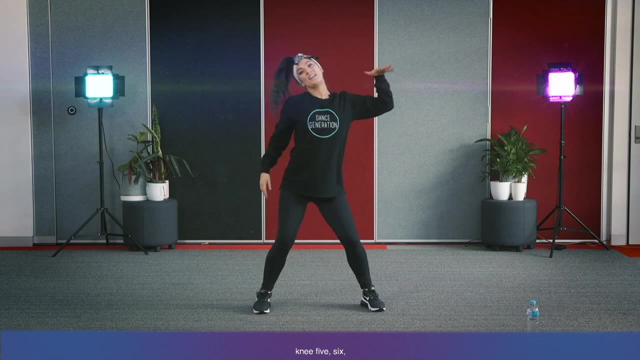 We're going to do that twice. okay, We just finished doing this one. I'm going to step out. I go one, two, three, four, knee five, six, jump seven, eight. We do it again. 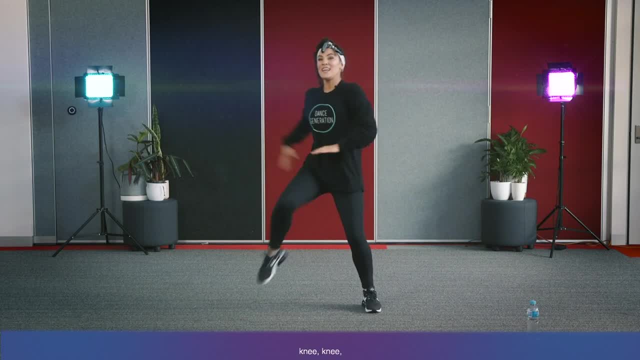 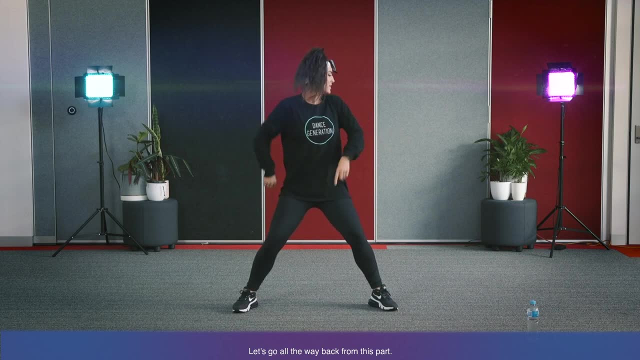 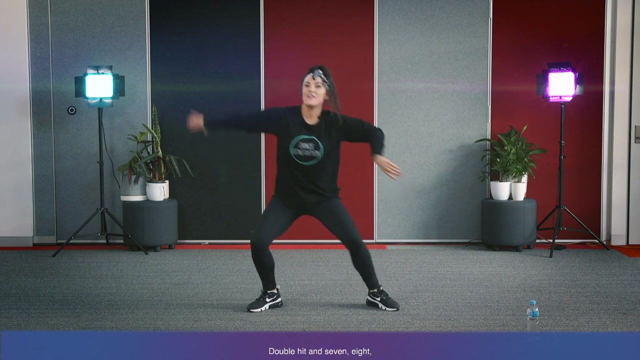 Fan yourself, Fan yourself, Fan yourself. Knee knee in out. okay, Let's go all the way back from this part. I did hit and hit, double hit and seven, eight. We go groove to the other side and groove to the other side. 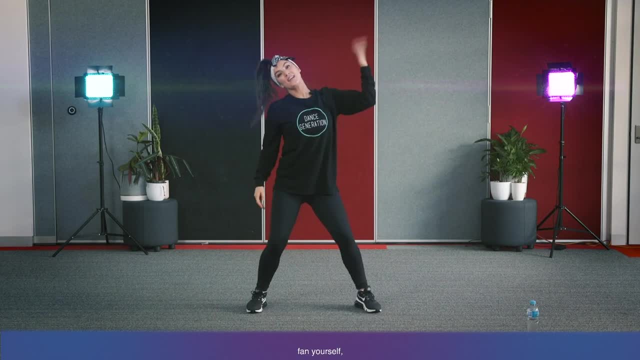 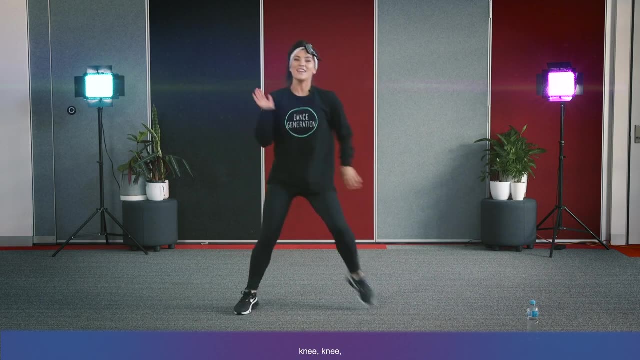 New part: Fan yourself, Fan yourself, Knee and knee And do it all again And fan and fan Knee, knee, in out. All right, let's keep going. We just did knee and knee and in out. 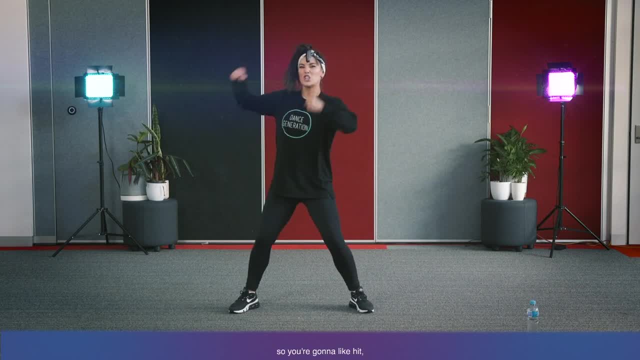 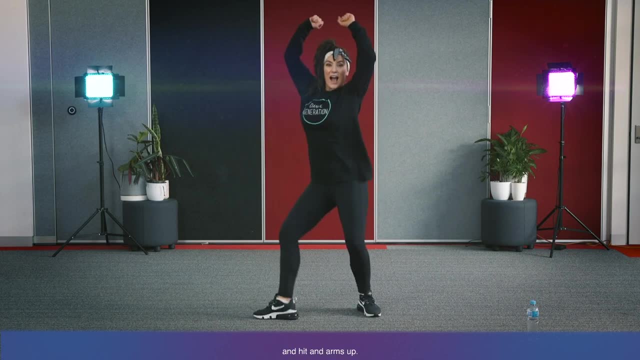 From here I want you to bring your knees up. You're going to go hit, So you're going to like hit, like either side of your knee. We're going to do both knees. We're going to go hit and hit and arms up. 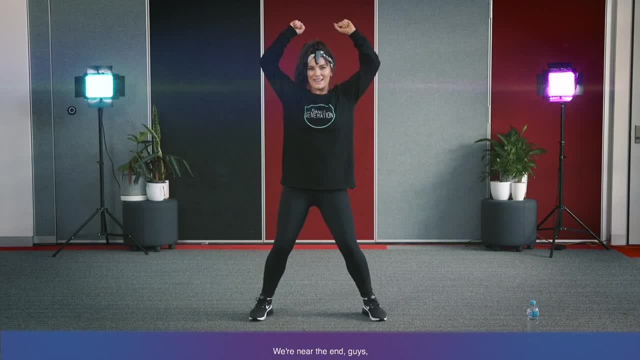 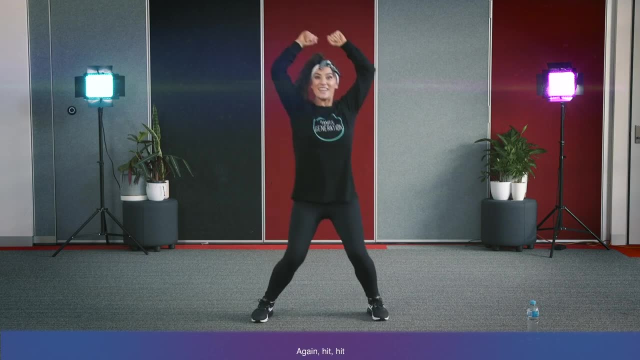 But this part, my heel is just coming through. We're near the end, guys, So we really want to give it all that we've got. You're going to go hit, hit and heel, heel again. Hit, hit and heel, heel. 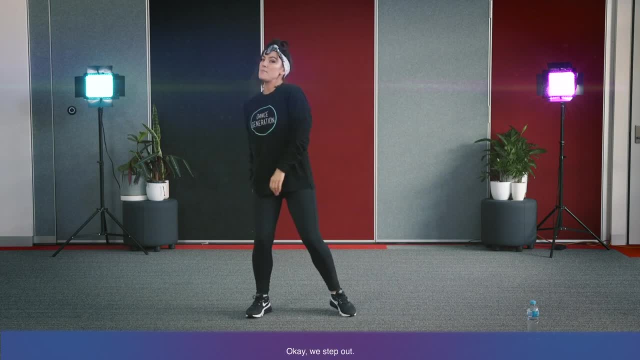 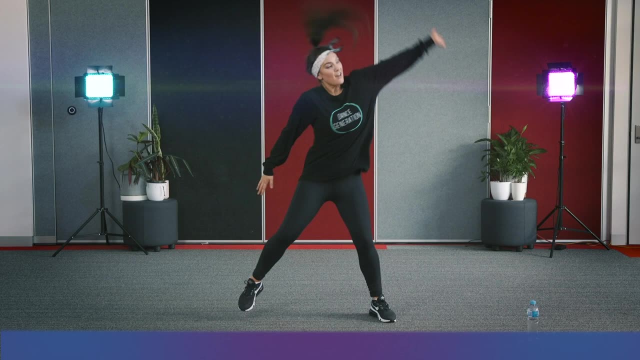 All right, Let's take it from the fan. Okay, We step out, Fan yourself, Fan yourself, Knee, knee. And do it again: Fan fan, Knee, knee and in, out And hit and hit And heel. 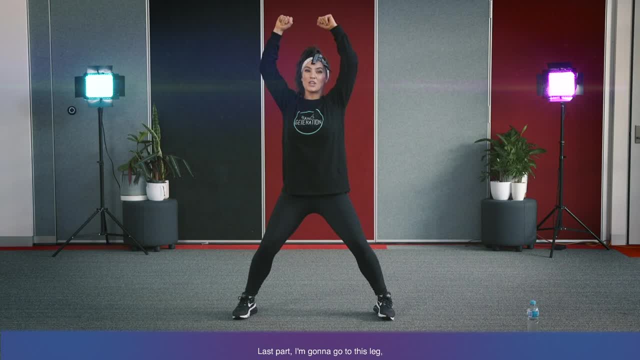 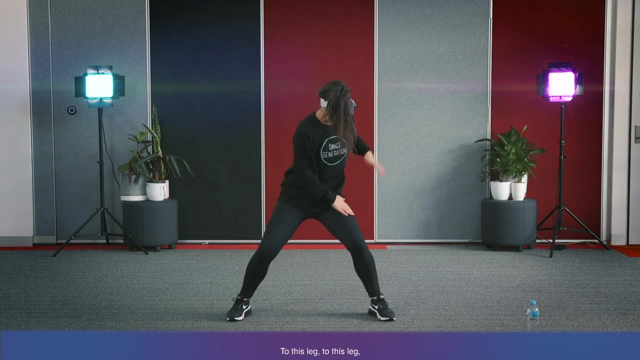 Hit hip and heels, Last part. I'm going to go to this leg, Two little steps, Bend your knees. I'm going to go one and two and three and four Ready To this leg, to this leg, to this chest up Again. This leg, this leg, chest up Faster. One and two and three, and. 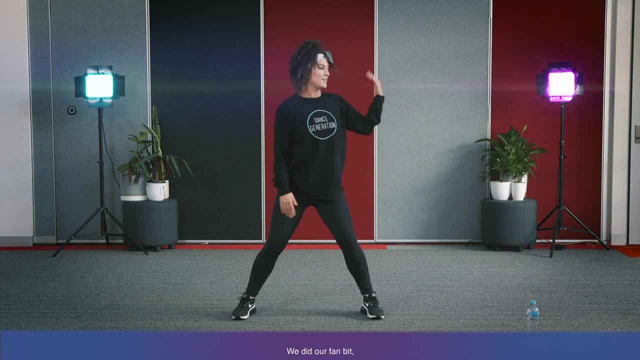 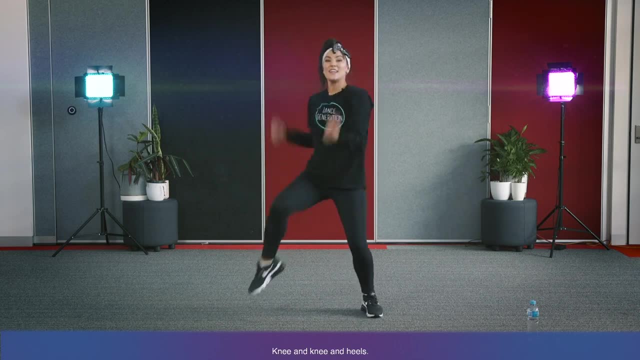 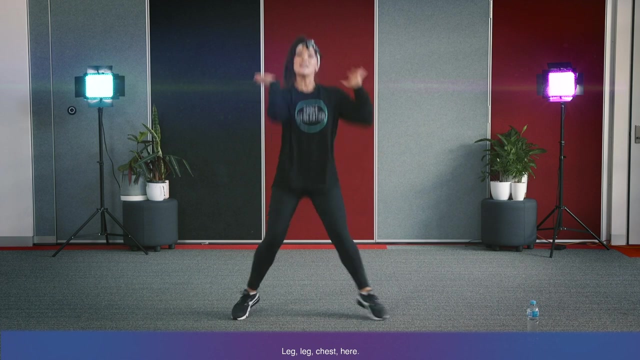 four: Okay, We did our fan bit, We did all this. We did the knees, Knee and knee and heels, Knee and knee and heels, to our leg, Leg, leg, chest, up Here, And then I want you to like, your knees are going to come up and your arms are going. 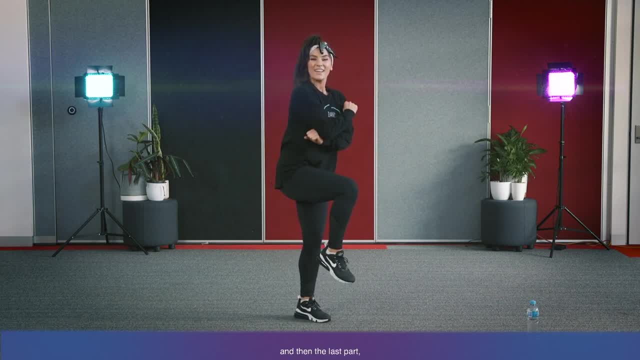 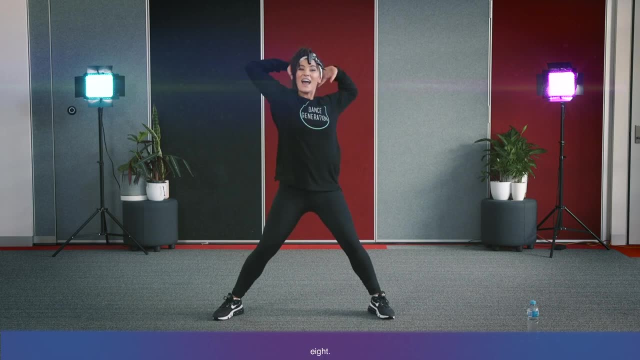 to scoop. That's on five. And then the last part, you get to do three poses of your own. You jump out, You've got six, seven, eight. It could be six, seven, eight Or six, seven. 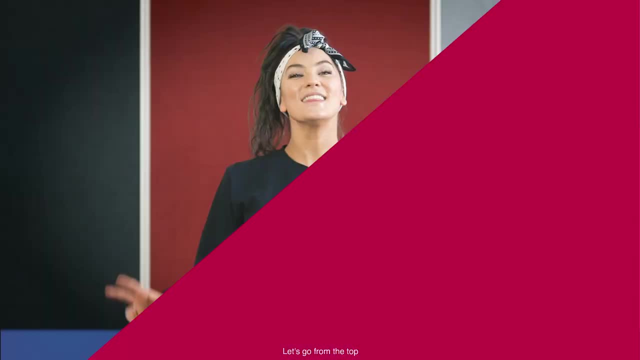 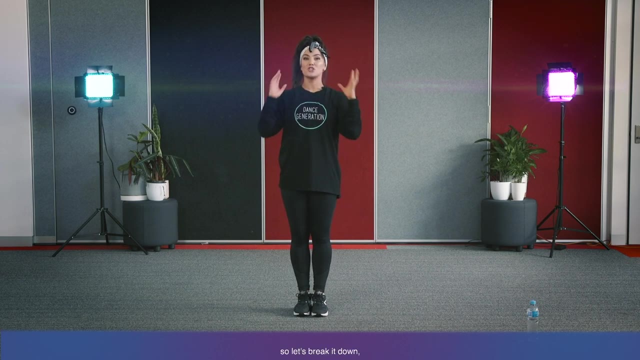 eight, Whatever you choose, And that's the end. Let's go from the top. Really slow, without music. You guys have finished the routine, But I know you're probably a little overwhelmed, So let's break it down. Do it from the top. 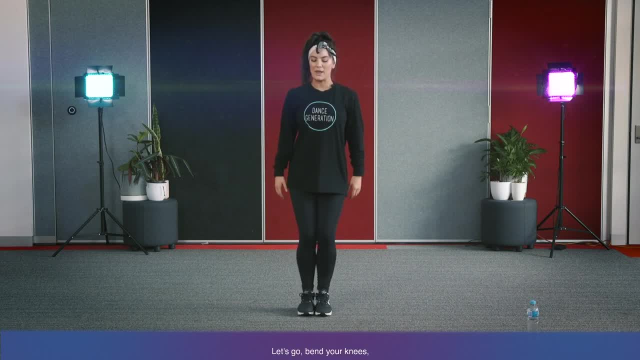 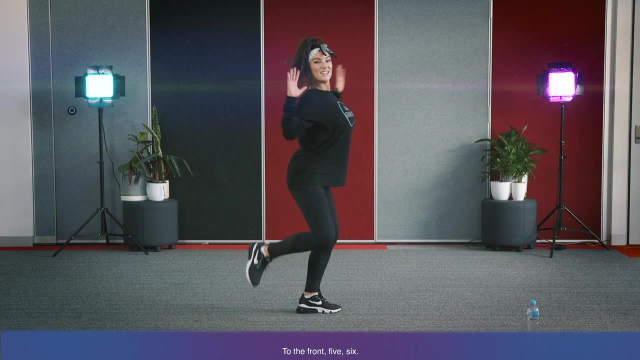 nice and slow, And then let's run it to music a few times. Let's go Bend your knees. We go Push it One, two To the side, Three, four To the front, Five, six, seven, eight. 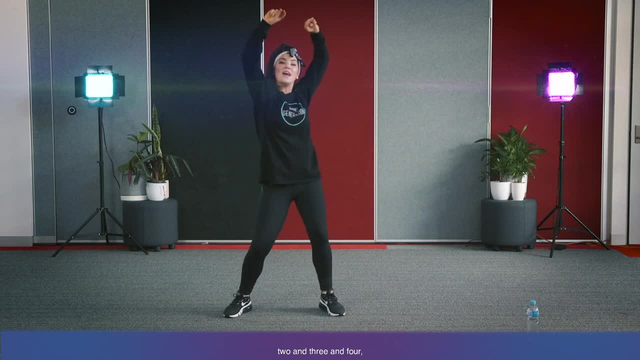 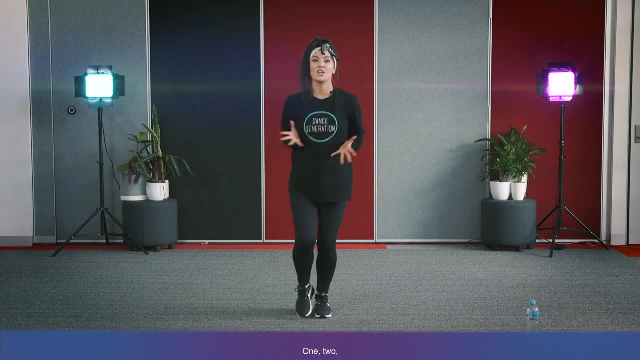 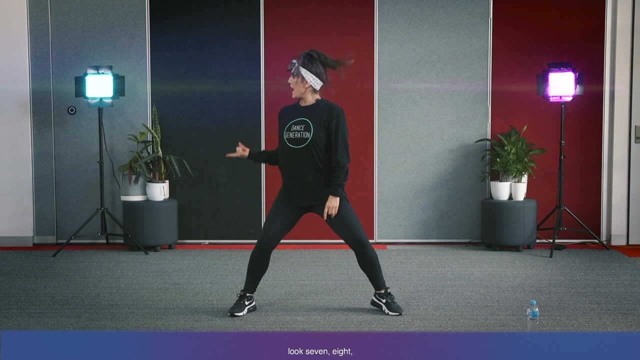 To the side One and two and three and four. Walk it out Five, six, seven, eight. Cross One, two, three, four, roll it five, six, look, seven, eight. punch it out one, two, three, four. 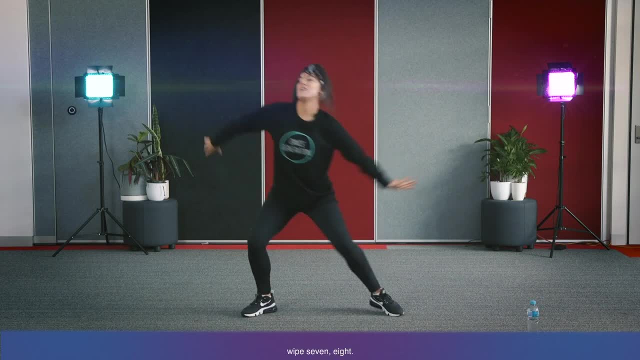 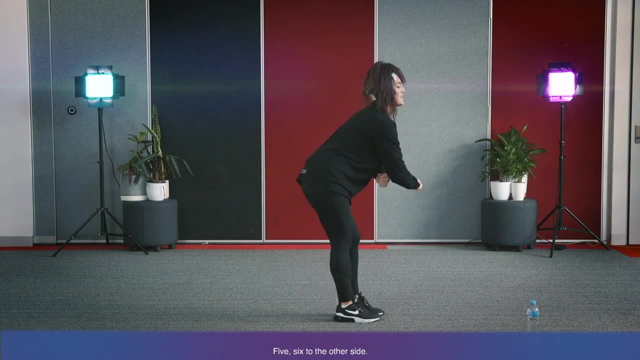 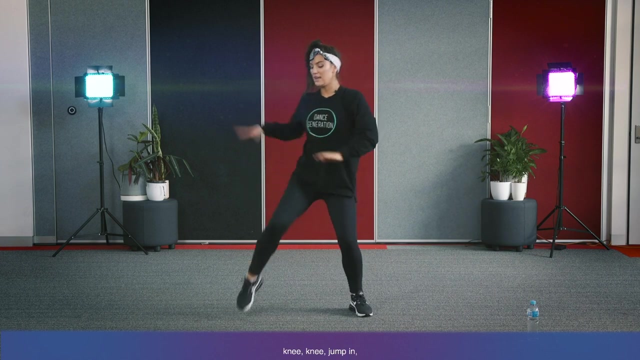 double hit: five, six, what seven, eight? we groove one, two to the other side, five, six to the other side. we go, fan ourselves, fan ourselves. knee knee, jump in let's. 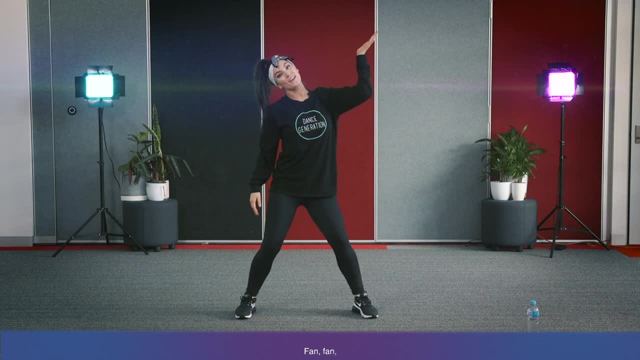 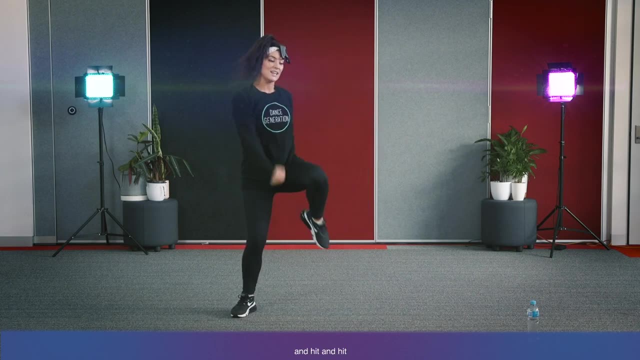 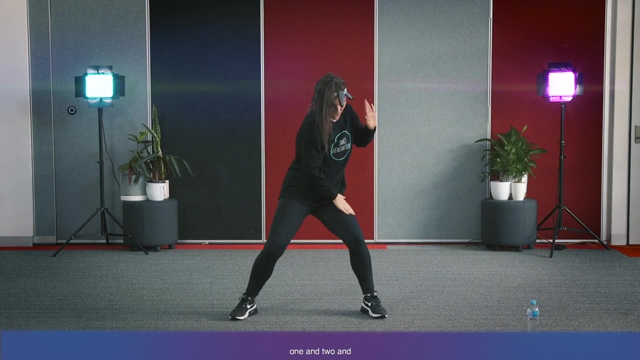 do it again. fan fan. this hand goes to your knee, knee, last pipe- and hit and hit and heels. and hit and hit and heels to your leg one and two and three. 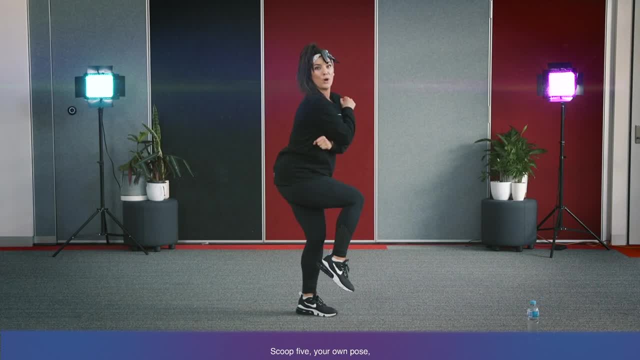 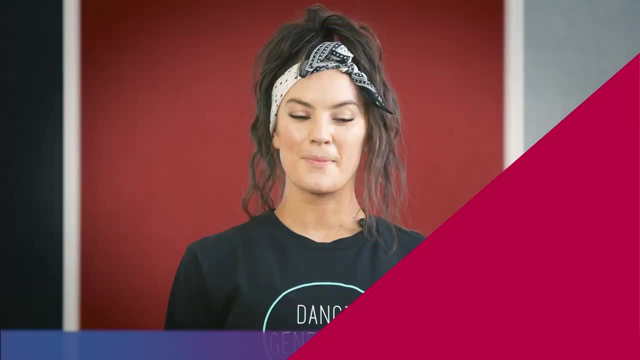 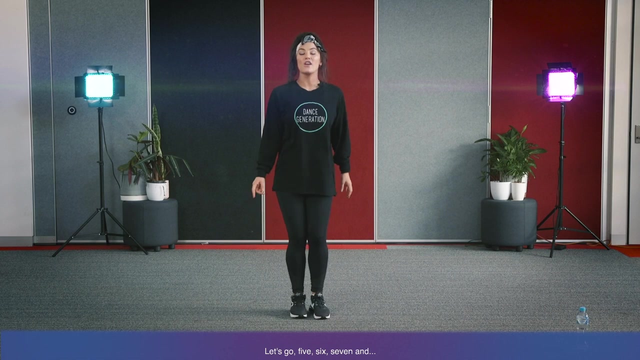 and four, go five, your own pose, six, seven, eight. that's done, let's roll it to music. All right, let's have some fun. let's go five, six, seven, eight. one, two, three, four, five, six, seven, eight. 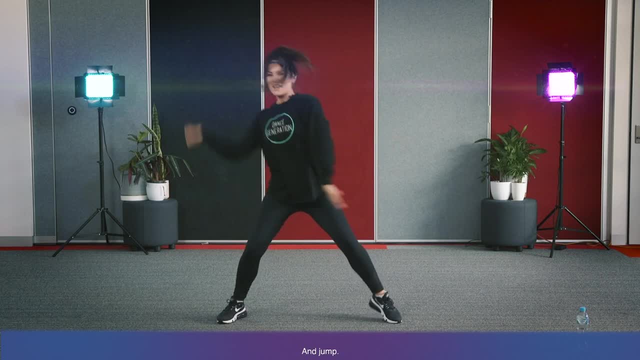 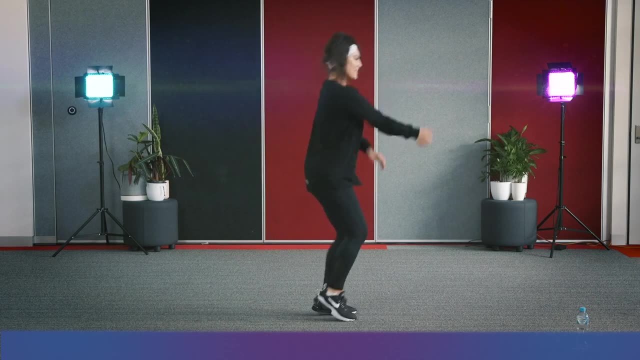 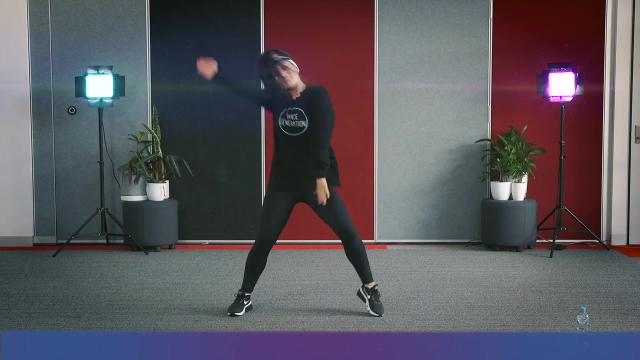 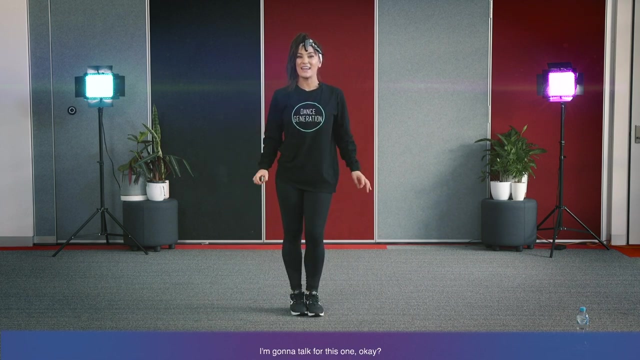 and jump and double punch, roll it to the other side, fan yourself and again: knee heel, knee heel, knee heel and jump and jump. I'm going to talk for this one, but on the last one I'm not going to do any talking. 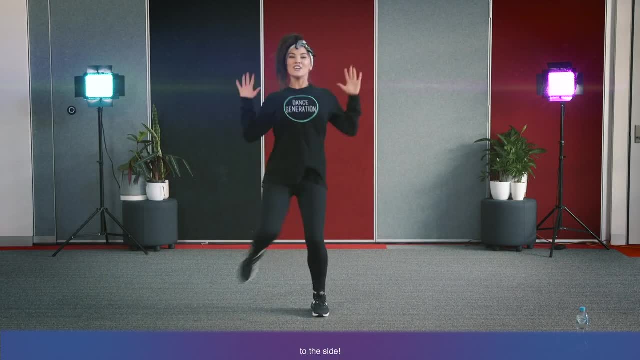 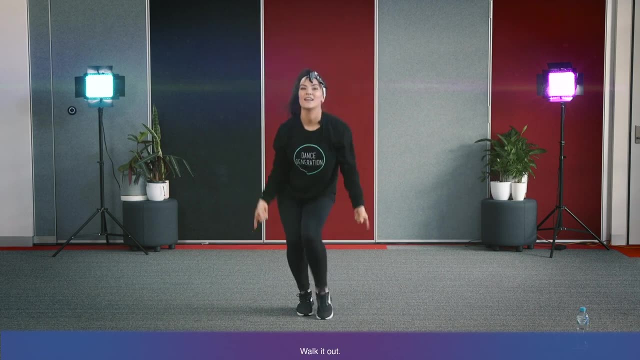 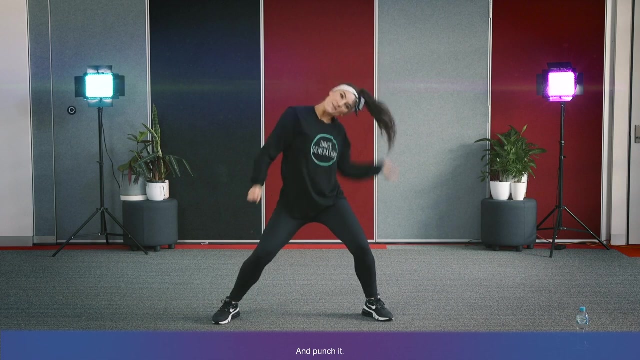 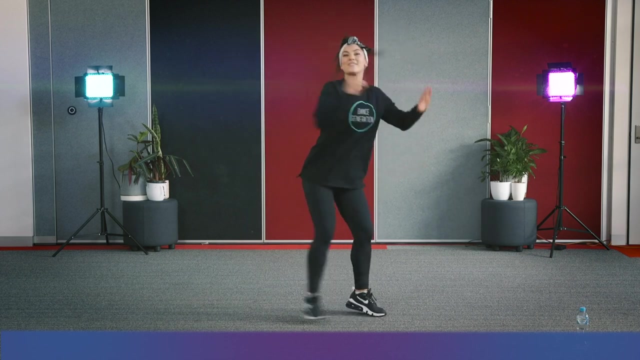 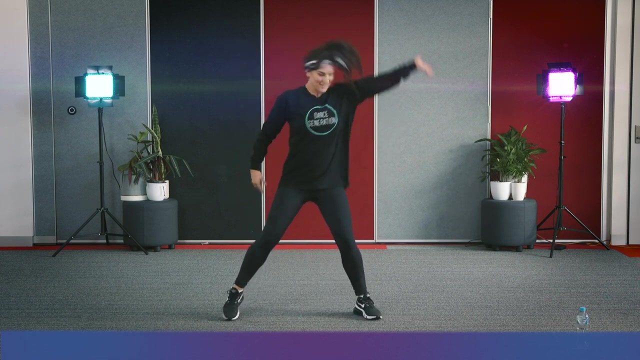 Let's go Five, six, seven to the side And push and bend your knees To the side, Walk it out And cross, Roll And punch it, Double punch. Let's groove it And bend And again.